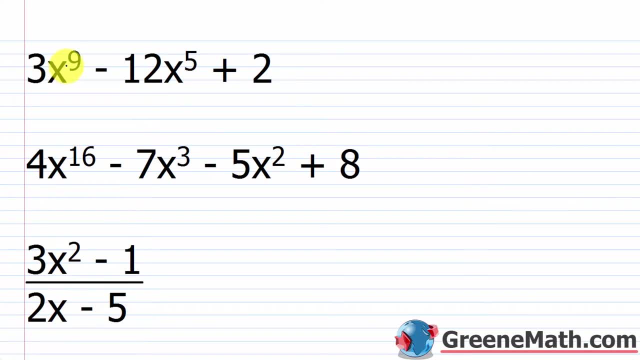 examples of a polynomial. so 3x to the ninth power minus 12x to the fifth power plus 2, this is a polynomial And all you're looking for is: on every term, do I have a variable where we don't have a whole? 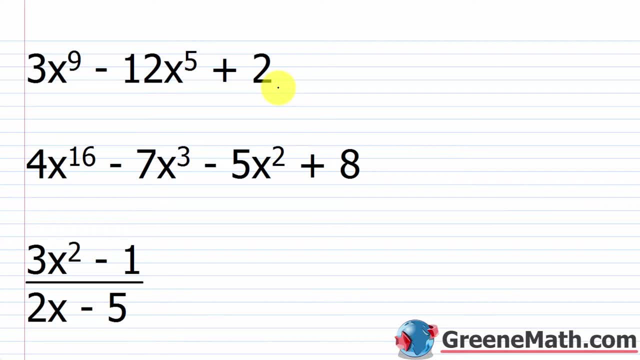 number as the exponent or where we have a variable in the denominator. If I look here, I have x to the ninth power and I have x to the fifth power. there's no variable in any denominator. so this is a polynomial, so we're good to go there. This one is another example. 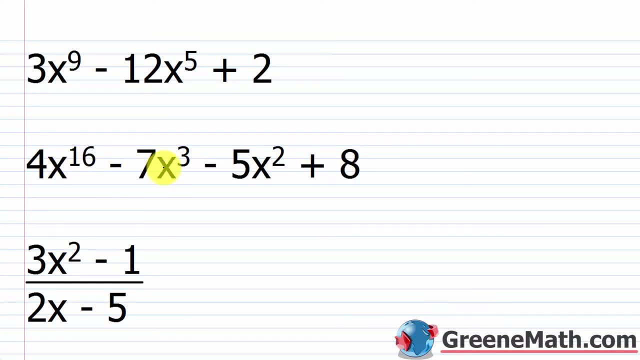 of a polynomial. we have 4x to the 16th power, minus 7x, cubed, minus 5x, squared plus 8.. So I look at my exponents here. I've got a 16,, a 3, and a 2, I'm good to go right. 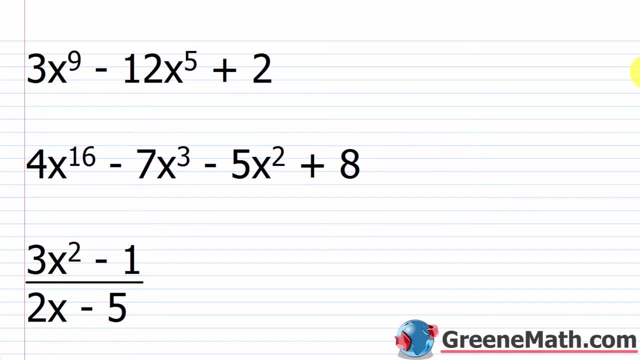 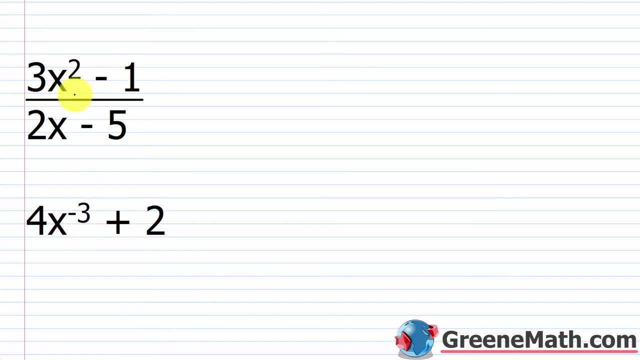 nothing is in the denominator. so we know that one is a polynomial. Now if I look at these two, they're not a polynomial. So 3x squared minus 1 over 2x minus 5 will have a variable in my denominator and that violates the definition of a polynomial. This is in fact called a rational. 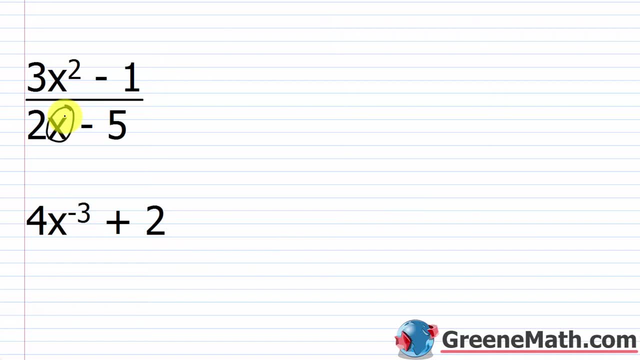 expression. right, we study those in Algebra 1, and we'll get to that in a little bit. So I'm going to look at my exponents here. I've got a 16,, a 3, and a 2,. I'm good to go right. nothing is in the. 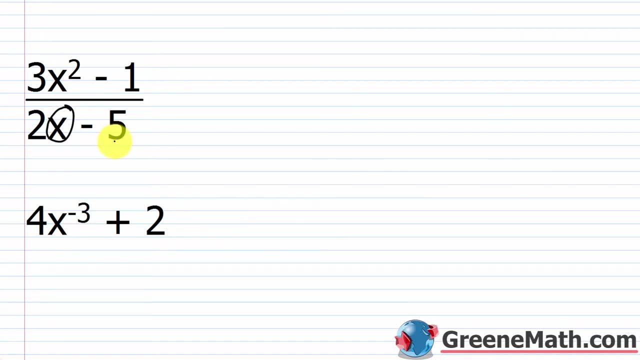 denominator. so we know that one is a polynomial. so we know that one is a polynomial. So I look at those pretty soon in Algebra 2, but this is not a polynomial. This other example here, 4x to the power of negative 3 plus 2, is also not a polynomial, because we have this exponent of negative 3.. So 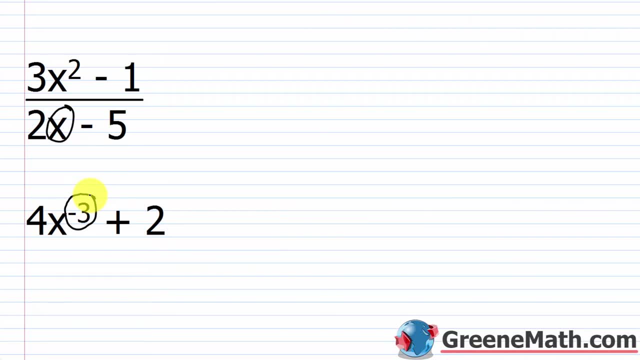 negative 3 is not a whole number. okay, if you see something like negative something, or you see a fractional exponent, something like that, you don't have a polynomial Again. your exponents have to be whole numbers only. All right, so we have three polynomials and we're going to look at them in. 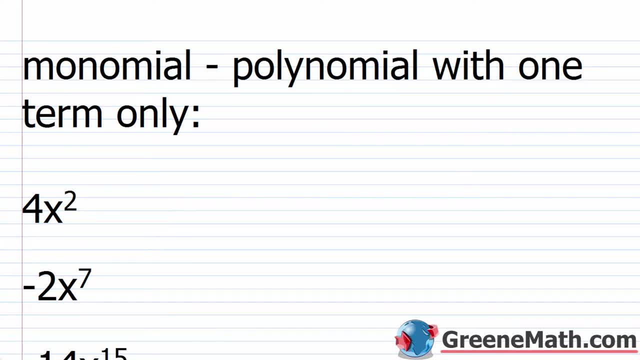 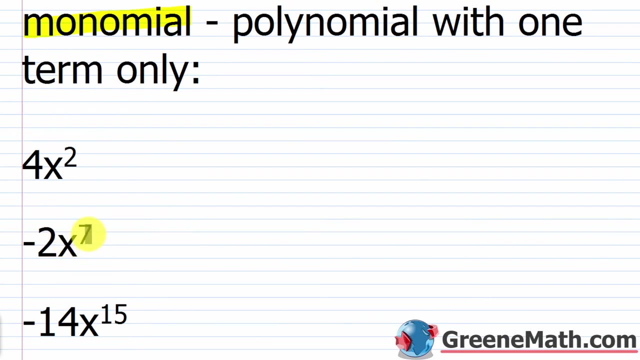 a little bit. So we have three polynomials that occur so often that we give them special names. The first one is referred to as a monomial. okay, so a monomial, So this is simply a polynomial with one term only. So three examples: we have 4x squared, so that's a monomial. negative 2x to the 7th power. 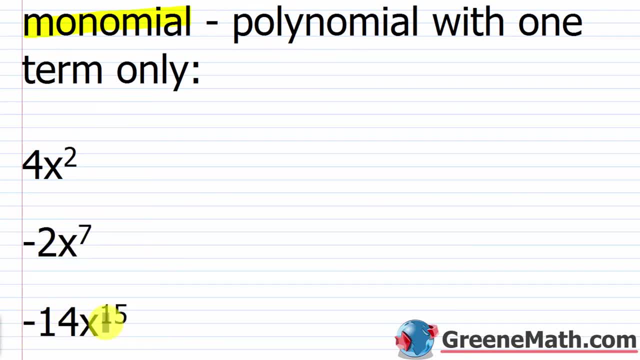 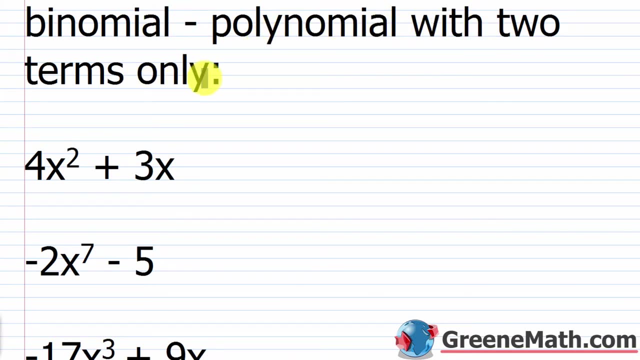 that's a monomial. and negative 14x to the 15th power, that's a monomial as well. So in each case we just have one single term, and that is the definition for a monomial. All right, so the next one would be a binomial. So this is a polynomial with two terms only. Now 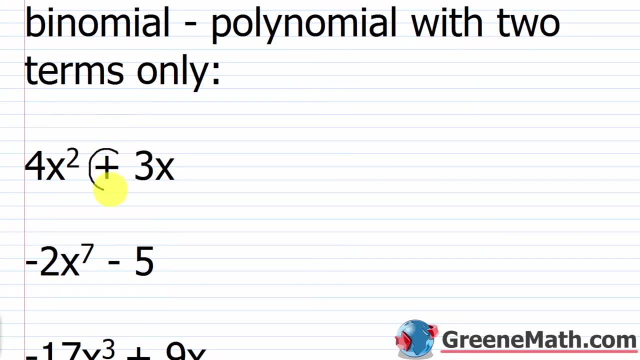 again notice how the terms are separated by either a plus or a minus sign. So when you see one of those signs, you know you've separated two terms. So this is a term and this is a term. So we've got two terms. in this polynomial I've got 4x squared plus 3x, so that is a binomial. Then the 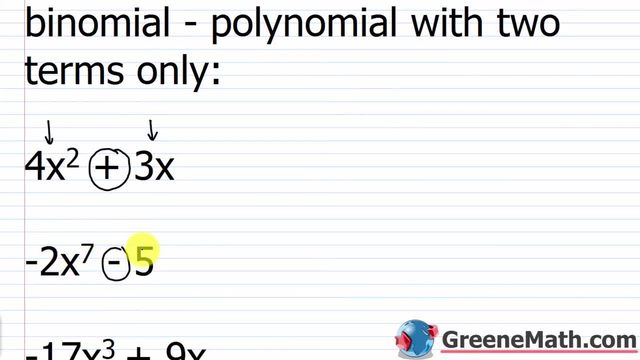 same thing here. I've got negative 2x to the 7th power- that's a monomial- and negative 14x to the 15th power minus 5.. So I've got a term here and a term here. The minus sign separates the two. So 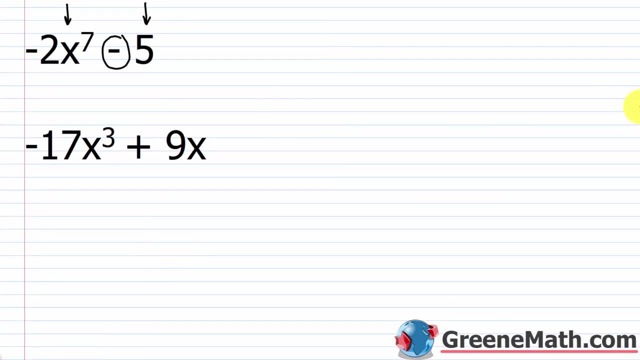 that's a binomial as well. And then, as a final example, I have negative 17x cubed plus 9x- Again, this is a term here. this is a term here. The plus sign separates the two, and so we know we have two. 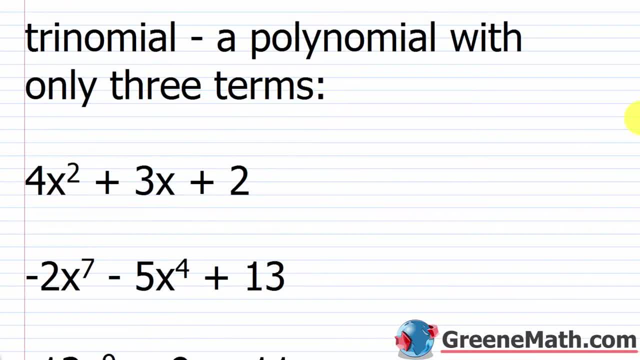 terms and that fits the definition of a binomial. All right, the next one we run across is called a trinomial. So this is a trinomial and this is a trinomial. So this is a trinomial and this is a. 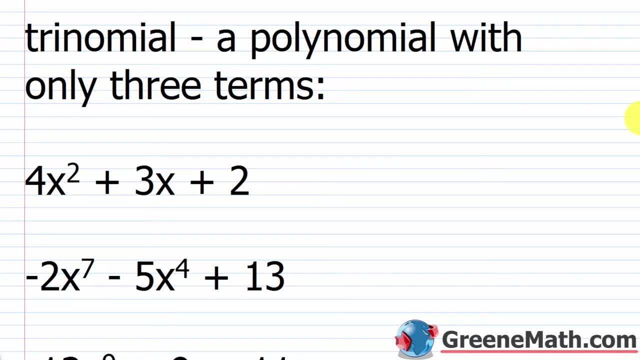 polynomial. Okay, we think about a tricycle has three wheels. A trinomial has three terms, So a polynomial with only three terms is a trinomial. So we have an example here: 4x squared plus 3x plus. 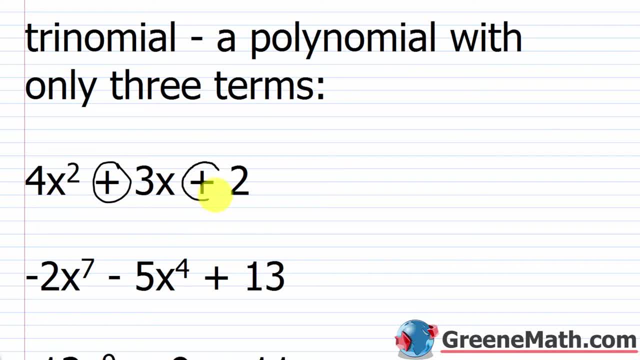 2. Again, everywhere you see a plus or a minus sign, you're separating terms. So you have a term here 4x squared, You have a term here 3x and a term here of 2.. So 4x squared plus 3x plus 2 has. 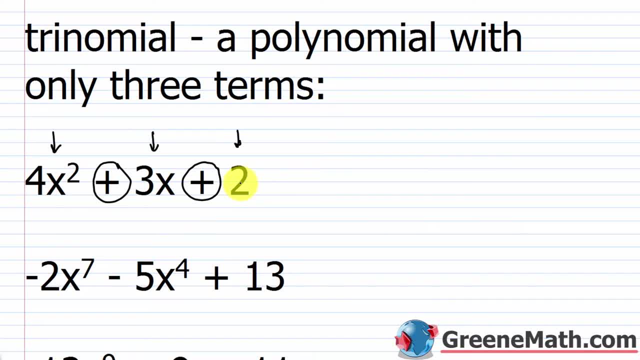 three terms and so it's a trinomial Same thing. here I have negative 2x to the 7th power minus 5x to the 4th power plus 13.. The minus sign and the plus sign separate the terms, So I've got a term here of negative 2x to the 7th power. 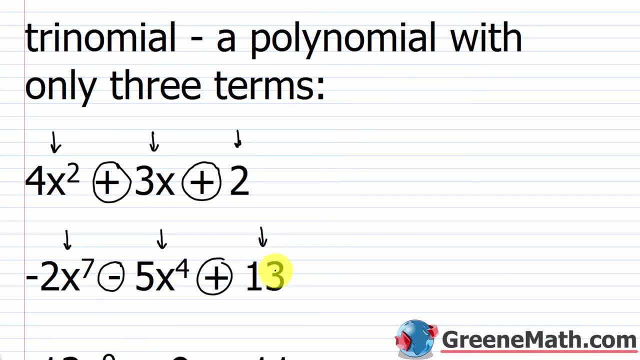 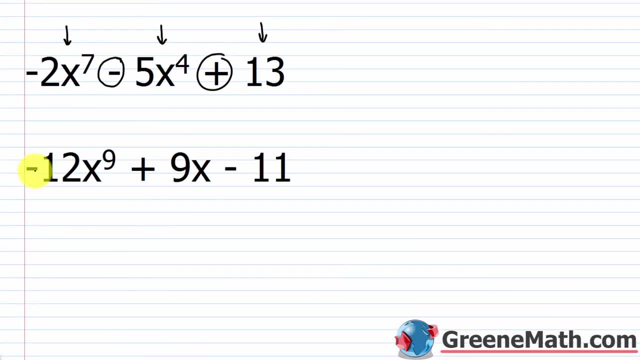 a term here of 5x to the 4th power and a term here of 13.. So we have a polynomial with three terms, and so that is a trinomial, All right. the last example is negative: 12x to the 9th power. 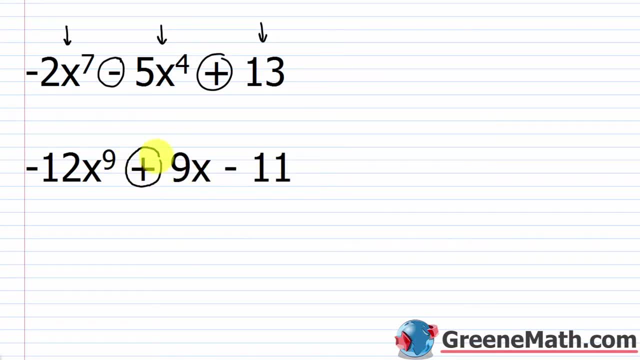 plus 9x minus 11.. Again, this and this plus and the minus separate the terms. So I've got negative 12x to the 9th power, I've got 9x and I've got 11.. So three terms here in this polynomial. So this is a trinomial, All right. 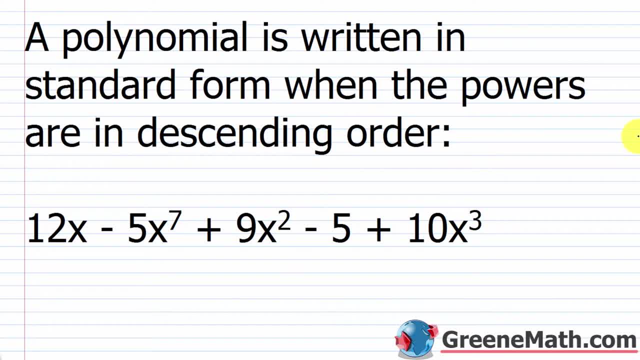 so pretty easy stuff overall, stuff that you would have learned in Algebra 1.. Here's another kind of common thing you need to know, and it's called standard form. So a polynomial is written in standard form. Let me just highlight that. So standard form When the powers are indecent. 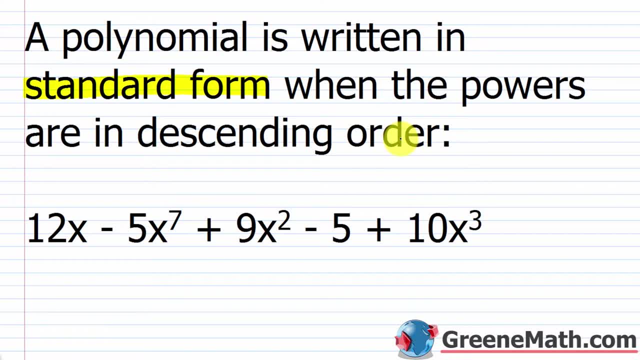 so this is starting all the way to the left and working your way to the right. So I'm going to take the term that has the highest exponent on the variable and I'm going to put it all the way to the left. Then I'm going to go to the next highest. 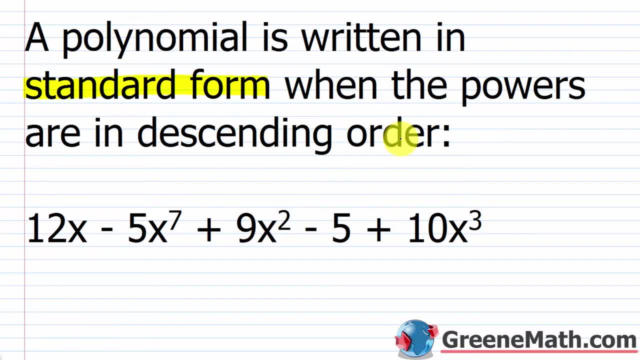 then the next highest, you know, so on and so forth. So if I look at this, 12x minus 5x to the 7th power plus 9x squared minus 5 plus 10x cubed, our variable is x. What is the highest exponent? 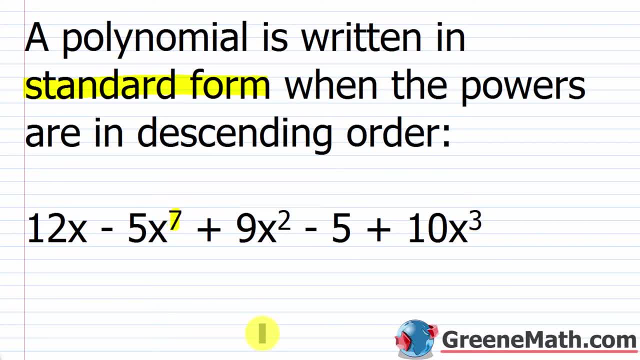 on this. So I'm going to put it all the way to the left. So I'm going to put it all the way to the 7th power. Well, it's this 7 here. So I want to write this term right here, and I've got to. 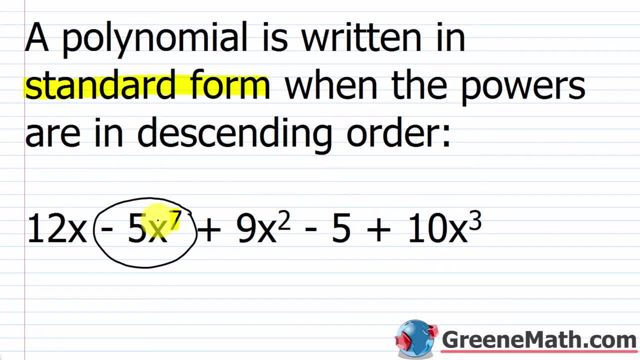 include that negative, the negative 5x to the 7th power. I want to put that all the way to the left. So if I put equals negative 5x to the 7th power, then I would say what is the next highest. 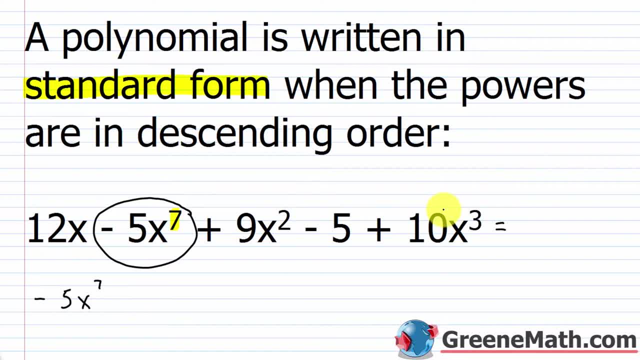 exponent. Well, this one's a 2,, this one's a 3, and this one's understood to be 1.. So I would go with this 3 here. So I'm going to put this 3 here, and I'm going to put this 3 here and I'm going to. 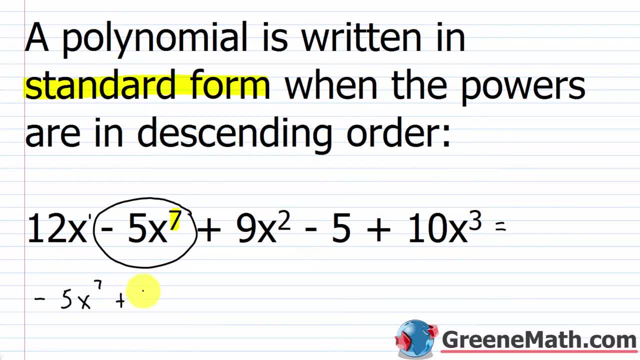 put this 3 here, So this term 10x cubed would come next. So plus 10x cubed, Then I'd put plus 9x squared, That would be next. Then I'd put plus 12x, That would be next, And then this constant. 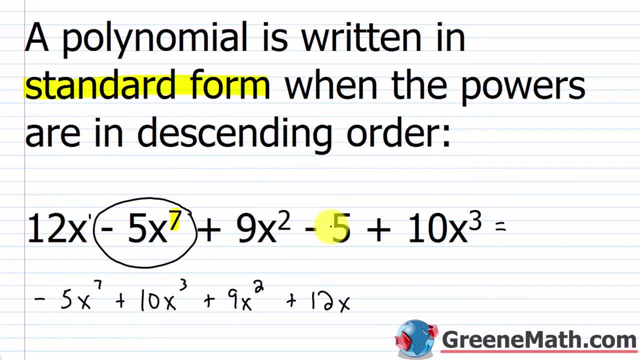 here. negative 5, would be all the way at the end. So this would be minus 5.. So this we could think of as being multiplied by x to the power of 0. You might see that in a textbook. I'm not going to. 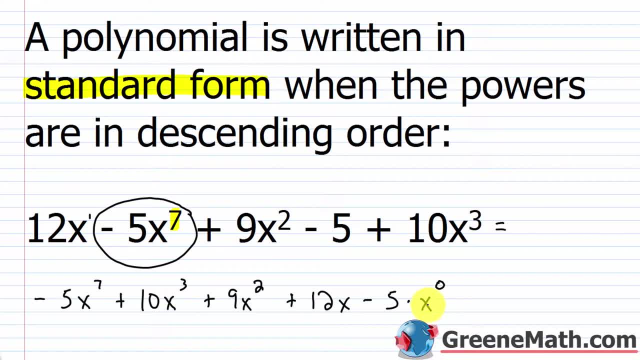 read that textbook and be very confused. You might say: well, why would they do that? So x to the power of 0 is understood to be 1, again, as long as x is not 0. So negative 5 times 1 is just. 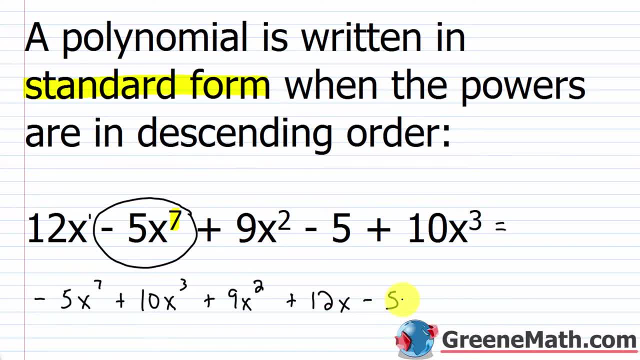 negative, 5.. So really I haven't changed anything there, It's just a neat little trick to put a variable next to it. So in standard form this polynomial is read as negative 5x to the 7th power. Notice how your exponents go in descending order. You've got 7,, 3, 2.. This would be a 1. And 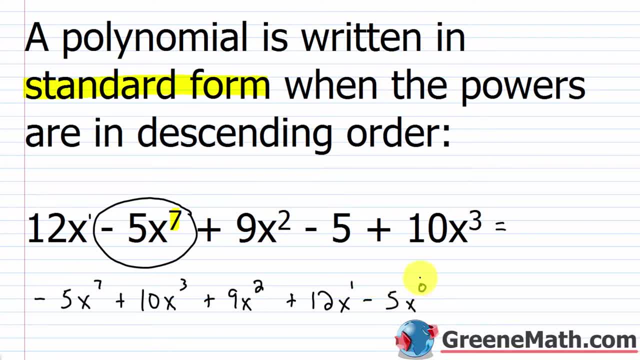 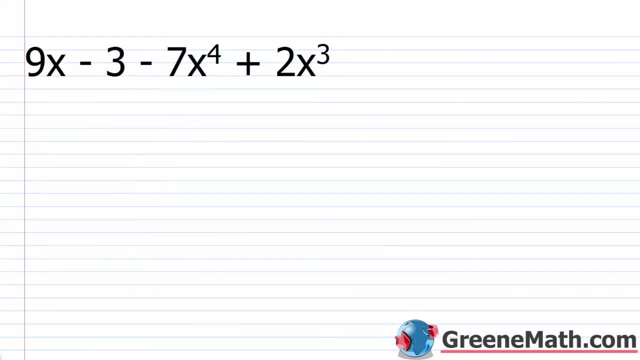 again. if you wanted to, you could write this as having an exponent on x of 0.. So 7,, 3,, 2, 1, and then 0. So in descending order, All right. so let's take this one and write it in standard form. 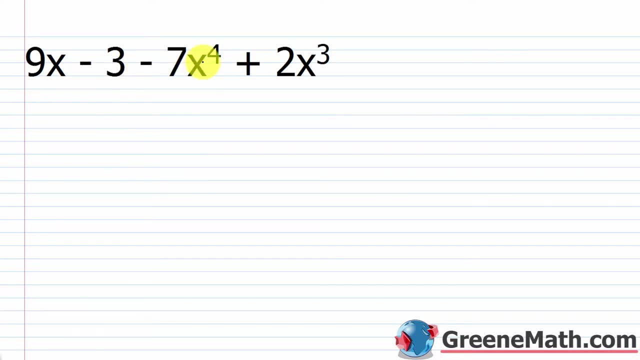 We have 9x minus 3, minus 7x to the 4th power plus 2x cubed, So the highest exponent on the variable here. So I've got to take that negative and bring it with me. So I'm going to put negative 7x to the. 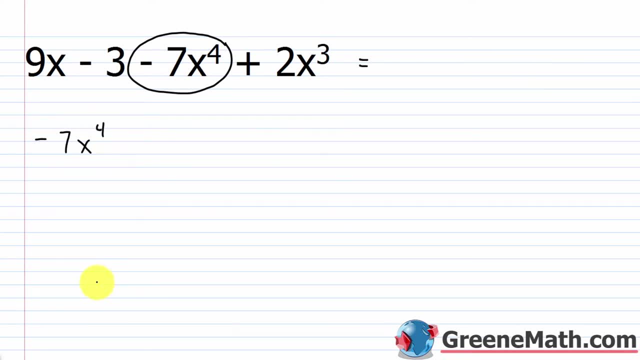 4th power. And you might ask yourself, if you're not familiar with a lot of things, why am I taking that negative with me? Remember, you can rearrange things with addition but not with subtraction. So if I put this as plus negative 7x to the 4th power, I just bring the negative with me. 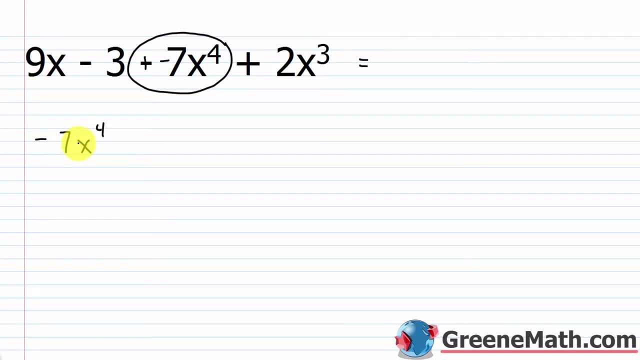 and I can rearrange things as much as I want. If I just took things as they were and I just moved this over here and I didn't put my subtraction over there and I just left the signs where they were, you'd have a problem there And 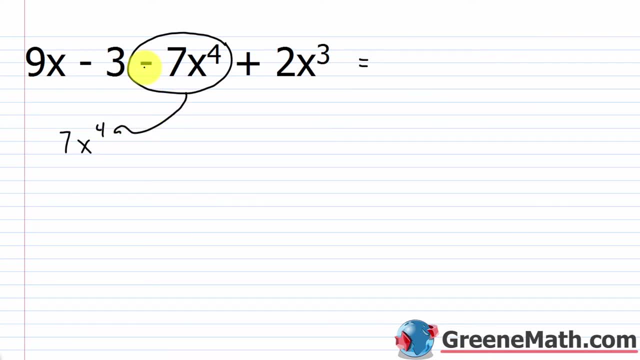 I can't just move this over here and leave the sign where it is. So I change this to plus negative and you can do it without doing it right. You can just mentally know that And just put a minus 7x to the 4th power, so there's no problems there. Now the next thing we want to think about is: 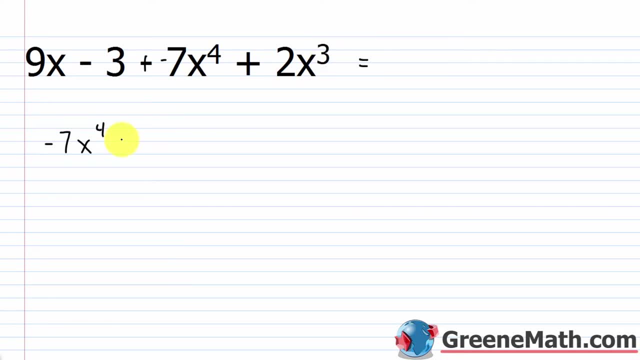 2x to the 4th power. So I'm going to put a minus 7x to the 4th power and I'm going to put a minus 7x cubed, right, Because the exponent there is a 3. So then, plus 2x cubed, And then next, 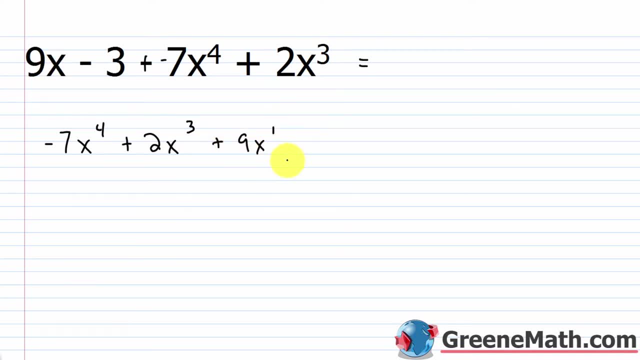 I want plus 9x, because the exponent there would be a 1.. And lastly, I just want that constant negative 3, or you can think about it as just minus 3.. All right, so I've rearranged everything. 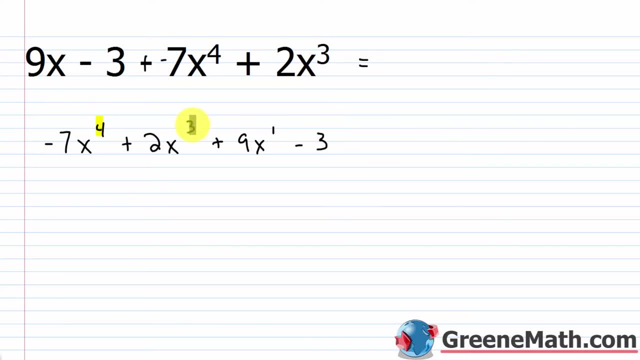 to where the exponents are in descending order. We've got a 4, a 3,, a 1.. And again you could write this as negative 3 times x to the power of 0. So then you could say you have a 0 here. 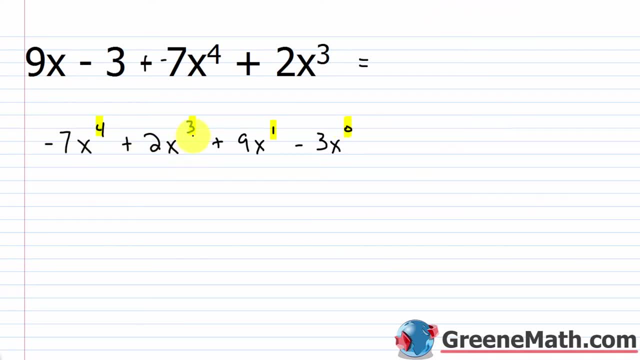 So negative 7x to the 4th power, plus 2x cubed, plus 9x, minus 3x to the power of 0. Or you could just put minus 3, right, Same thing. So the last thing we're going to review is called the degree. 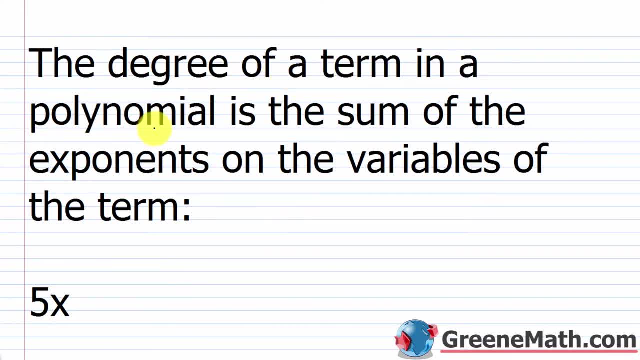 So the degree of a term in a polynomial is the sum of the exponents on the variables of the term. So all I'm going to do to find the degree is look at the exponent, or it could be exponents if you have more than 1.. So I'm going to look at the exponents and I'm going to look at the exponents. 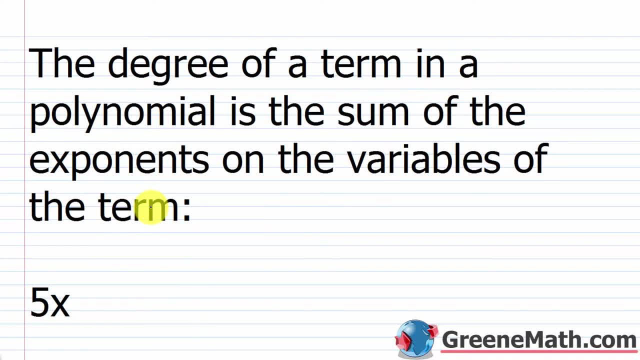 of the variable And whatever the sum is, that's the degree of the term. So in other words, with 5x- we know the exponent here is understood to be 1. So the degree is 1. For this example. 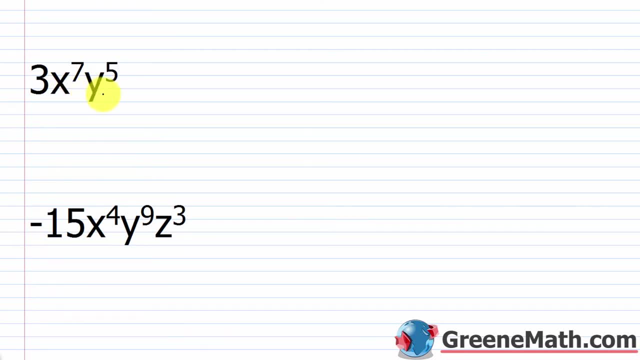 3x to the 7th power, y to the 5th power. we have two variables involved, So what I want to do is some addition. I have an exponent of 7 and an exponent of 5.. 7 plus 5 is 12.. So the degree. 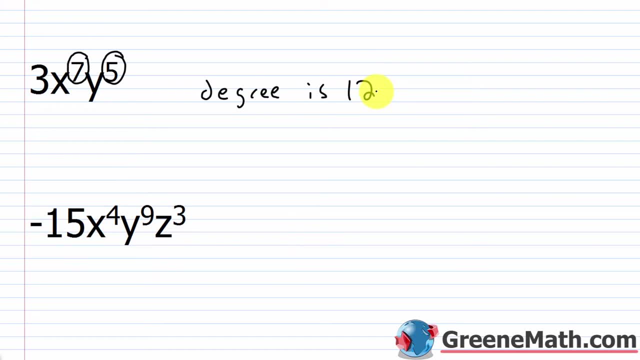 is 12.. So this isn't very difficult at all. It's just something you just kind of need to know, right? Once you know it and you understand the definition, it's very, very simple, right? Just some simple addition For this one negative 15x to the 4th power. 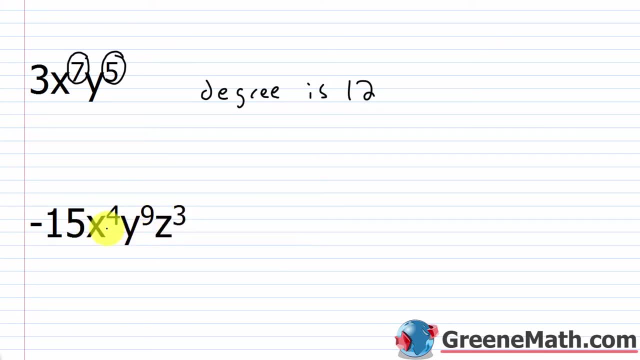 y to the 9th power, z cubed. Again, I'm just going to add the exponents. So 4 plus 9 is 13.. 13 plus 3 is 16.. So this plus this, plus this, your degree. 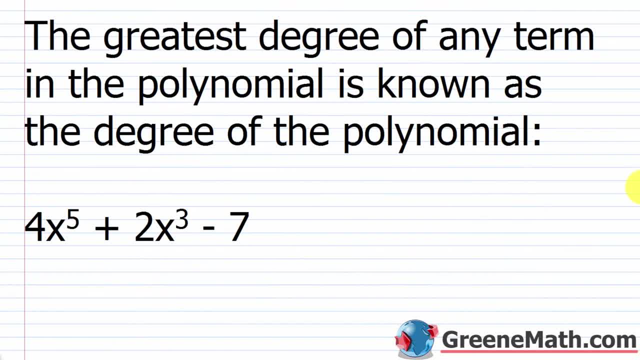 is 12.. Alright, so let's extend this a little bit further. Now we're going to talk about the degree of the polynomial itself. So the greatest degree of any term in the polynomial is known as the degree of the polynomial. So as an example here I have 4x to the 5th power plus 2x cubed. 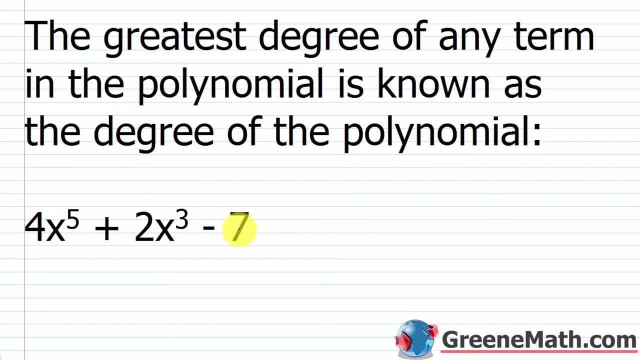 minus 7.. So I would look at each term individually. So for this term here, the exponent is 5.. So the degree of that term is 5.. Then this term here, 2x cubed, the exponent is a 3. So the degree of the term is a 3.. And then for this negative 7, again, 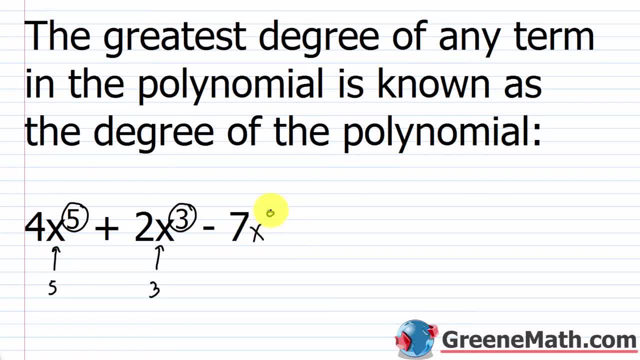 a little trick here. I can write x to the power, of 0 next to it. I showed you that earlier. So the degree for this would be 0.. Now which term has the highest degree? Well, this one does the 4x to the 5th power. So since the degree for that term is a 5, that means the degree of the. 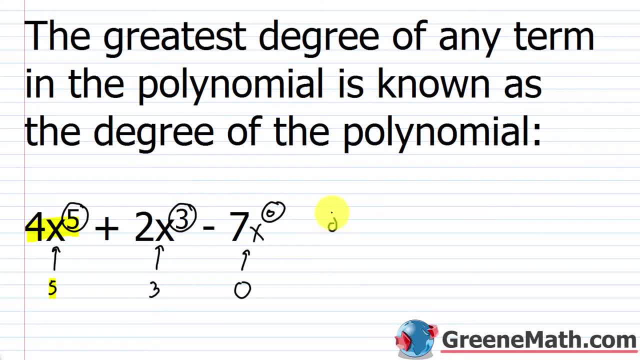 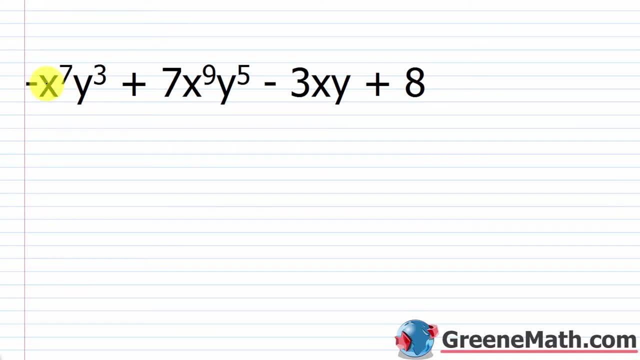 polynomial is a 5.. This polynomial has a degree of a 5. So the degree of the polynomial is a 5.. All right, let's take a look at another one. So we have negative x to the 7th power, y cubed. 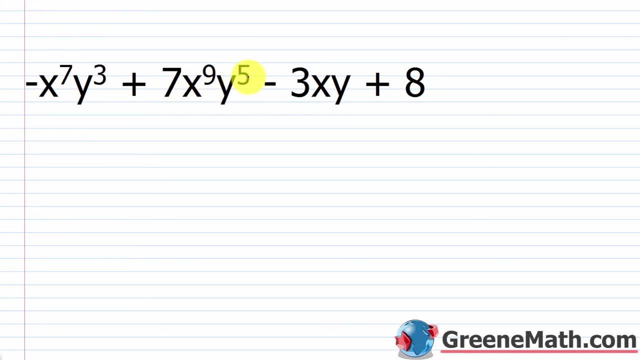 plus 7x to the 9th, power y to the 5th minus 3xy plus 8.. So again, I want to look at each term individually. to start, If I look at this term here, I have a 7 as an exponent and a 3. I've 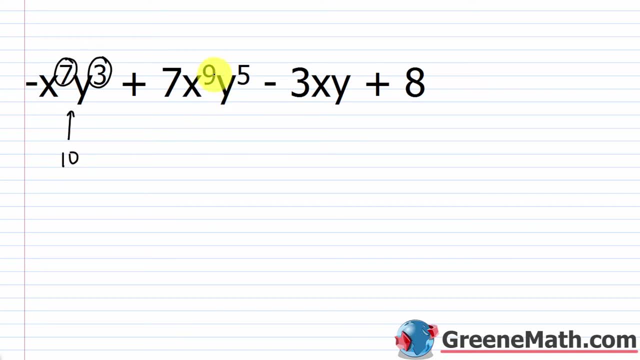 got to sum those two. So 7 plus 3 is 10.. For this one I have a 9 and a 5.. 9 plus 5 is 10.. 5 is 14.. For this one I have a 1 and a 1.. 1 plus 1 is 2.. And then for this 8, here I can write this: 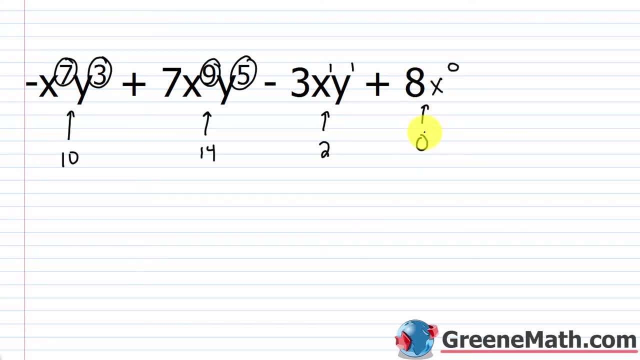 as times x to the power of 0. So this is 0.. In general, when you look at a constant, the degree is 0. Now, the only exclusion to that is the number 0 itself, But anything other than 0,. 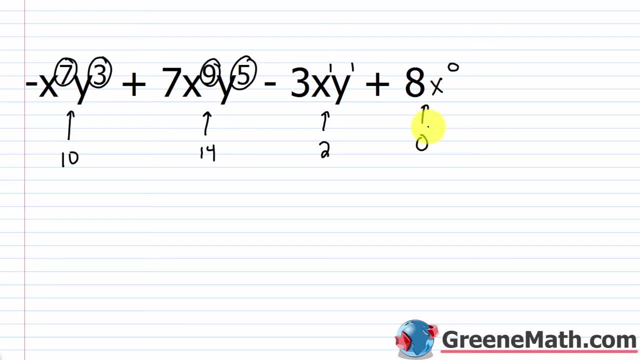 if it's a constant, it's going to have a degree of 0. So if I think about this polynomial here, we see that this is a 0. So if I think about this polynomial here, we see that this is a 0.. 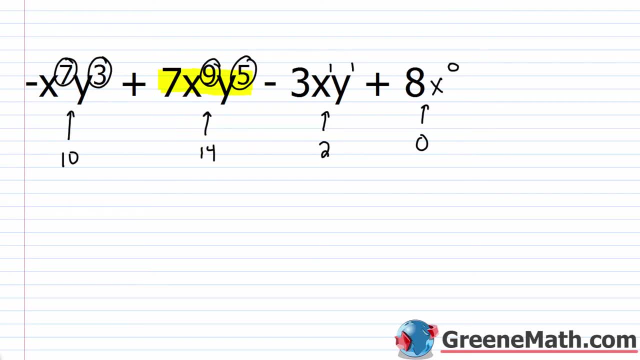 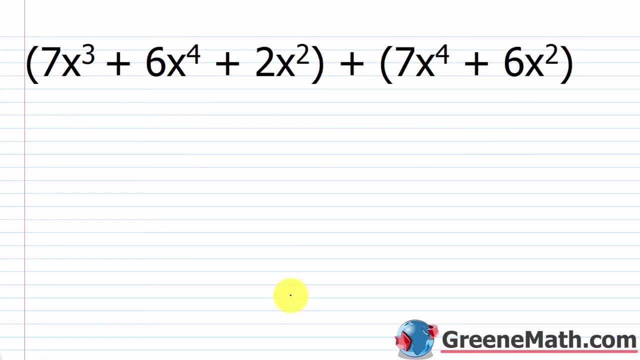 This is the big winner here this term, right here. So the degree for this is 14.. So the degree for the polynomial is 14.. So the degree is 14.. All right, so now that we've kind of reviewed some of the things that we need to know, let's jump in and start adding and subtracting. 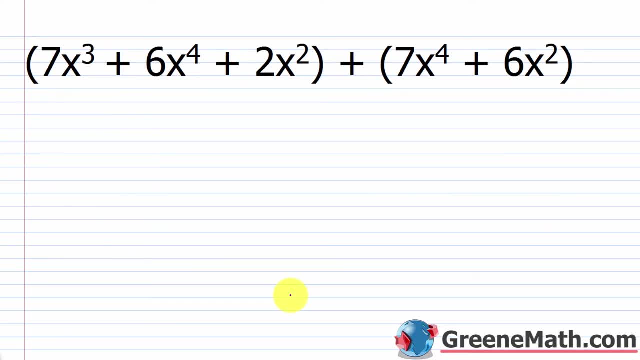 polynomials. So for the majority of you, you've already done this. This is a review And you remember how easy this is. The only thing you have to really get down here is the concept of like terms. So like terms have the same variable, or it could be variables if we have. 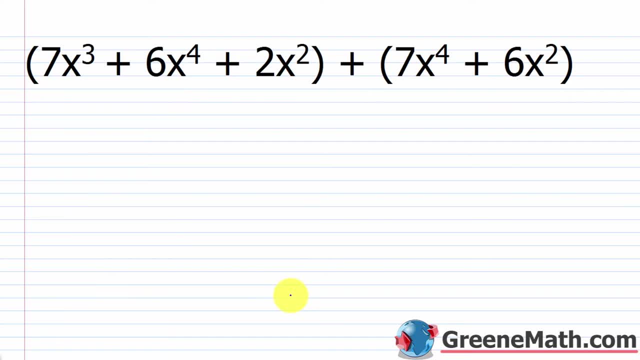 a harder problem And they're raised to the same power, or it could be powers. So, as an example, if I have something like 2x to the third power and I have 3x to the third power, those are like terms, The coefficients or the number parts here don't matter, Don't pay. 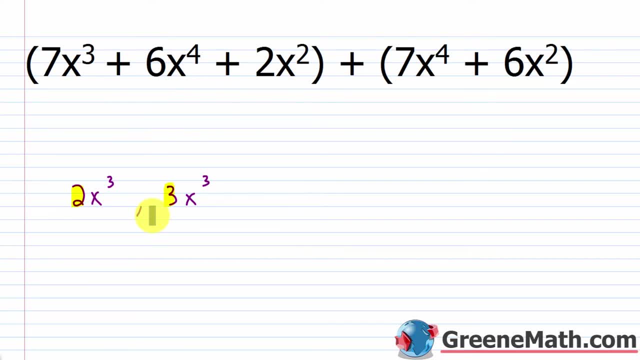 attention to that when you're trying to find like terms. I just want to make sure that the variable is the same. So I have an x here and an x here, So that's good to go. Then I want to make sure my exponent's the same. I have a cubed. 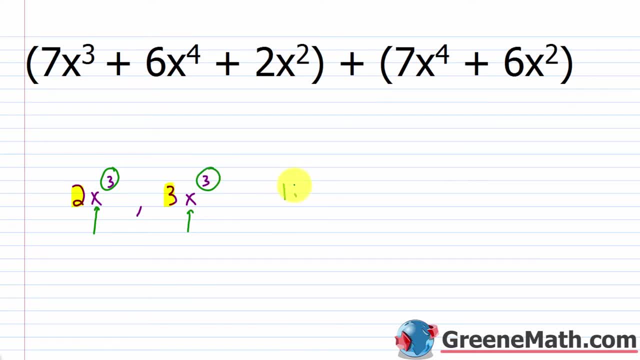 and I have a cubed, So that's the same. So these are like terms. And how do we go about adding like terms? Well, if I had something like 2x cubed plus 3x cubed, all I need to. 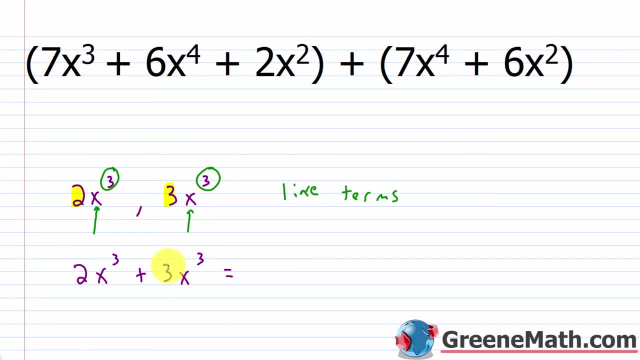 do is add the numerical coefficients, So 2 plus 3. Which is 5. And then the x cubed part stays the same Times x cubed. You can think about it as having 2 apples plus 3 apples gives you 5 apples. But if I wasn't adding like terms, let's say I was. 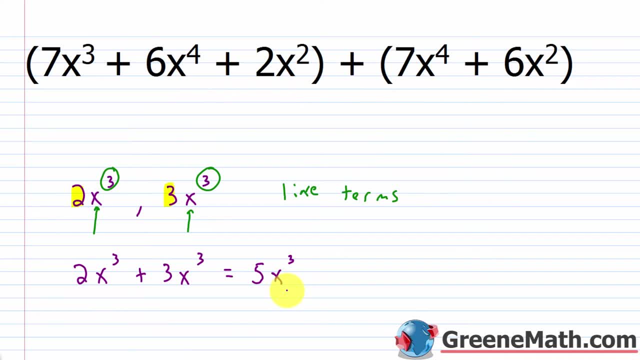 adding oranges and apples. Well, 2 apples plus 3 oranges is just 2 oranges and 3 apples. I can't really make that simpler. So as an example of something that's not like terms, let's say that I have a cubed here And let's say 3y to the fourth power. Well, these are not like terms. 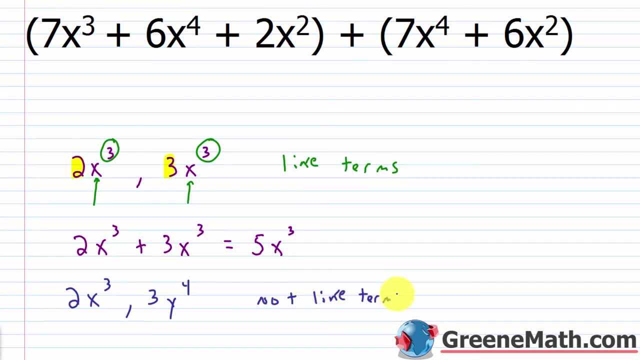 These are not like terms. Why is that the case? Well, I have an x here and I have a y here, So the variables are different. The exponents are also different. I have a 3 here and a 4 here. But even if the exponents were the same, it doesn't matter. It needs to be. 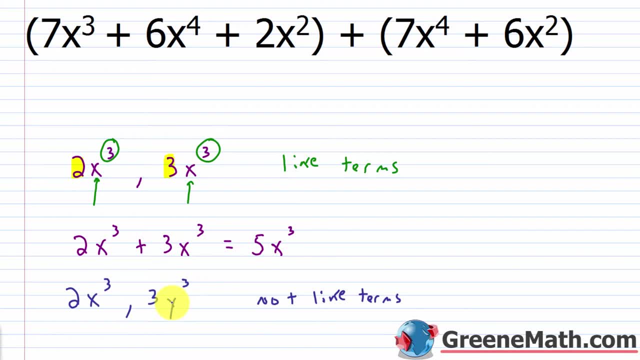 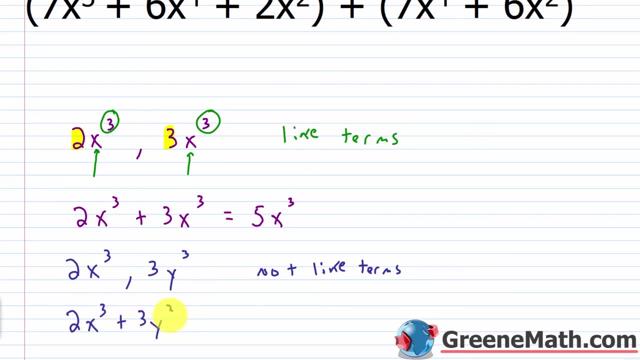 the same variable raised to the same power. Okay, so that's how you have like terms. So if I added 2x cubed and 3y cubed, you can't combine that or make that any simpler. There's nothing you can do And a lot of students make the mistake and say, okay, this is 5x cubed y. 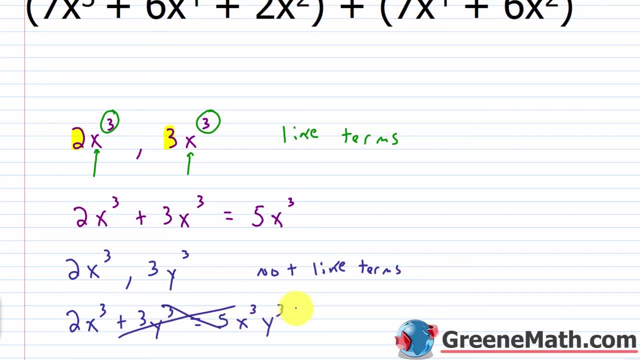 cubed. You can't do that. That's wrong. Okay, this is wrong. So very important that you understand that. you can only combine like terms. All right, so let's erase all this. I think all of you pretty much understand that. So let's erase all this. I think all of you pretty much understand. 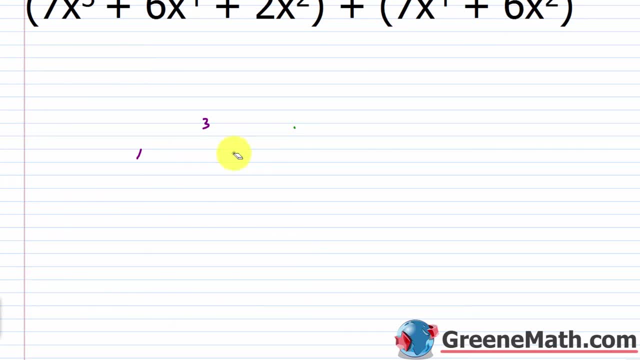 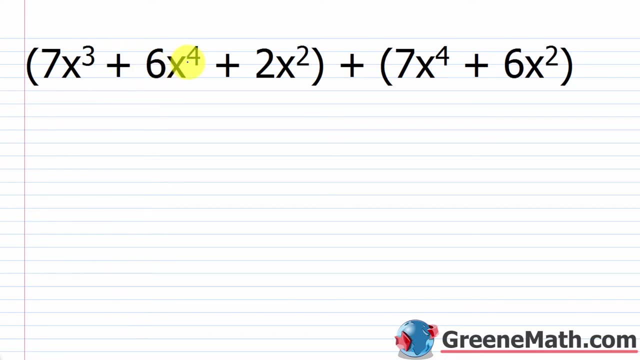 this at this point. If you don't, as we're working through the examples, I think you will easily pick this up. So I start out with adding this polynomial here: 7x cubed plus 6x to the 4th power, plus 2x squared, And we're adding to this the other polynomial, 7x to. 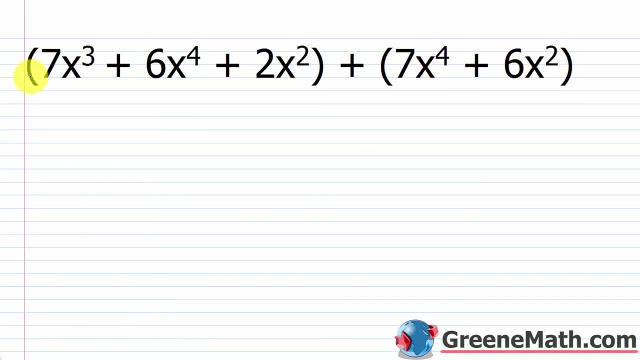 the 4th power plus 6x squared. The first thing is I can just drop these parentheses. I don't really need them, So I can write this problem as 7x cubed plus 6x to the 4th power plus. 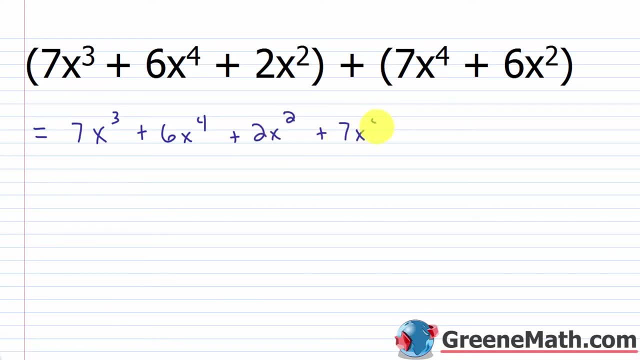 2x squared plus 7x to the 4th power, plus 6x squared. Now the next thing that I like to do- and I don't do this anymore, but when I started, my teacher told me this and I loved doing it- 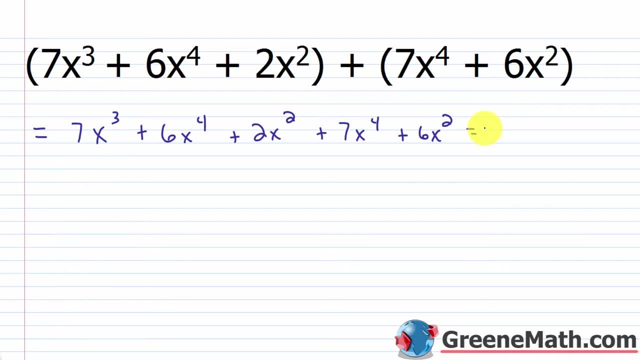 when I was struggling. I want to look for like terms right away and I want to write them next to each other, so it's obvious what I need to do. So in other words, if I start out with 7x cubed, 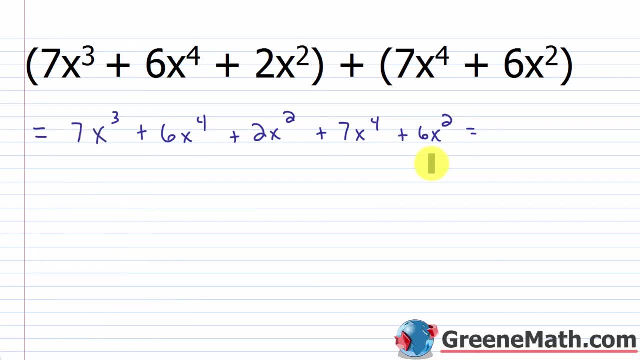 do I have another term with an x cubed in it? No, I do not, So I don't need to do anything. I have 6x to the 4th power. next, Do I have another term where I have x to the 4th power? 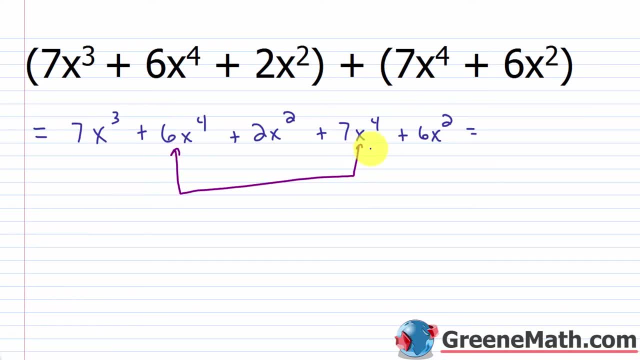 Yeah, I have this one and this one. Then I have 2x squared. Do I have another term with x squared? Yeah, this one and this one. So let's reorder this. I'm going to put 6x to the 4th power in the very front position, then plus 7x to the 4th power, then plus 7x cubed. 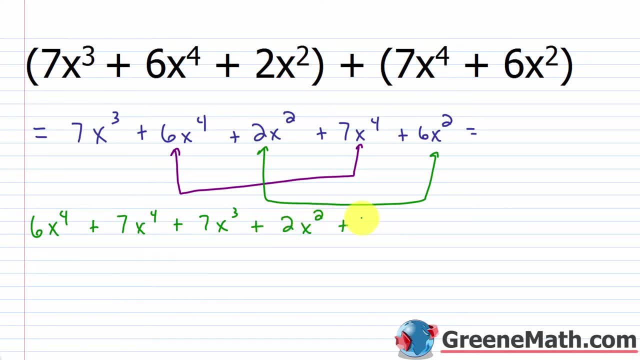 then plus 7x to the 4th power, then plus 7x to the 4th power, plus two x squared, then plus six x squared. Now I did two things there. The first thing is I took the exponents that were highest and move them to the left, And I went in descending order. So 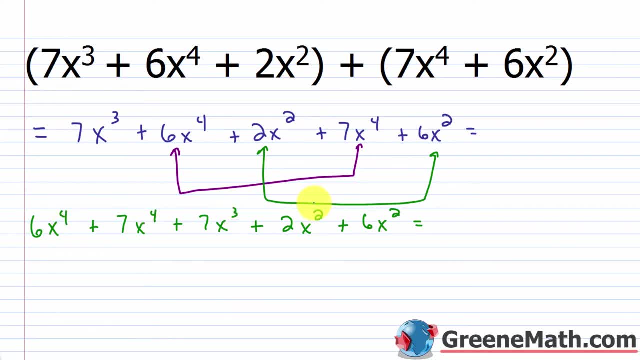 this is the exponent with a four, a four, a three, then a two, then a two, So it's in descending order. So when I get my answer it's going to be in standard form. Okay, so that's the first thing. 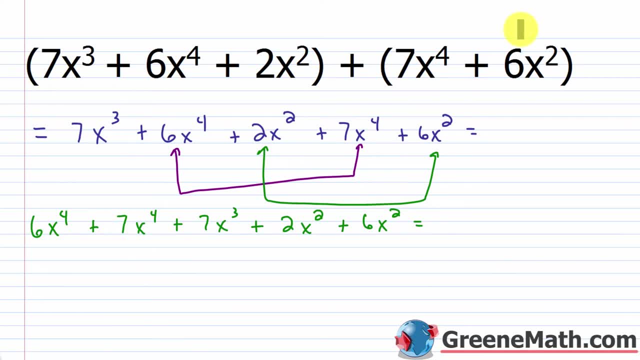 I did. The second thing I did was I arranged it to where like terms were next to each other. So these are like terms and these are like terms. So now all I got to do is add the coefficients, keep the variable part the same. So six x to the fourth power plus seven x to the fourth power. 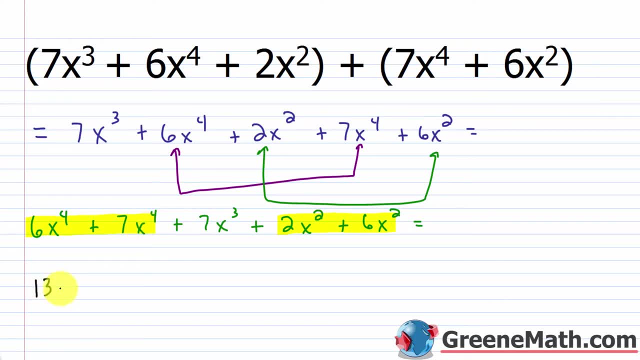 add six plus seven, that's 13.. And x to the fourth power just stays the same. If I had six apples and seven apples, I added them, I would have 13 apples. So then plus we have seven, x cubed. 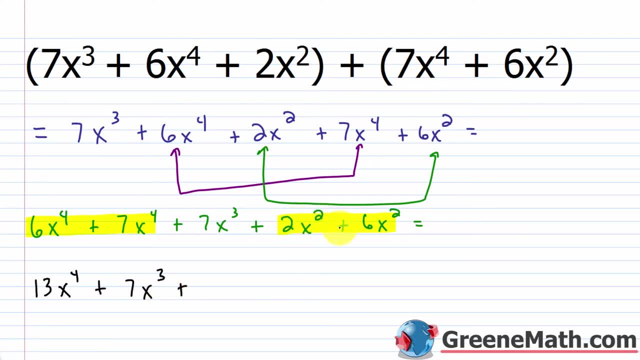 And then plus. now we have like terms again. we have two x squared plus six. x squared, two plus six is eight, And then x squared comes along for the ride. Now, there's no way to make this any simpler. We simply don't have any more like terms. Our variable is the same in each case. 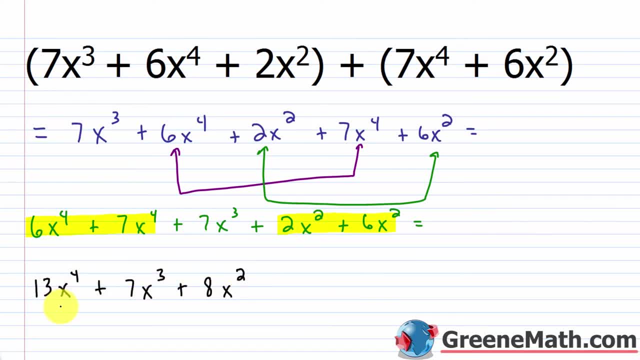 but the exponents are different. This is like adding apples, oranges and nectarines. Okay, if I had 13 apples plus seven oranges, plus eight nectarines, I can't really make that simpler. But I can just say: comes to me. if I said I have 13 apples and seven apples, I can just làve 20 apples. 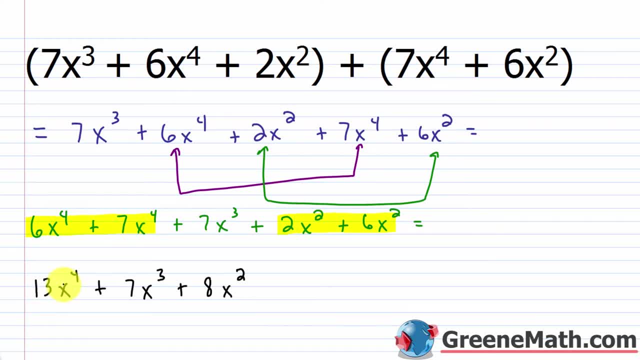 So that is kind of a real world example of what we're going through here. So our answer is just 13 x to the fourth power, plus seven x cubed, plus eight x squared. again, notice how it's written in standard form: You have x to the fourth, x cubed and then x squared, All right. 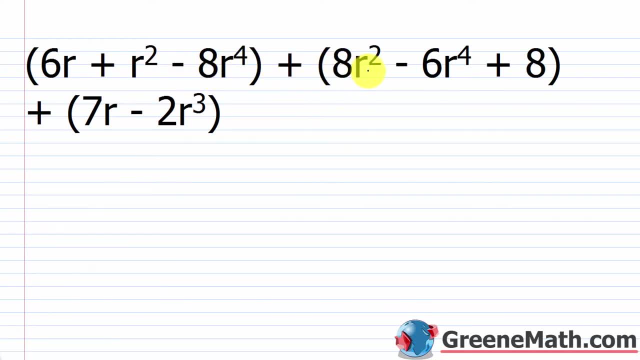 as the next example, we have six r plus r, squared minus eight r to the fourth power, then plus, Then plus. we have 7r minus 2r cubed. All right, so the first thing I want to do again is reorder these things. 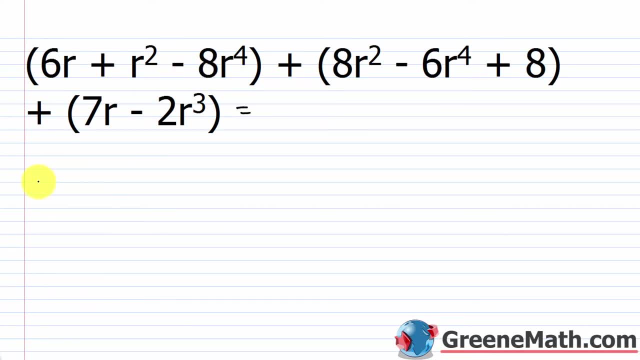 I'm going to start out with negative 8r to the fourth power. So negative 8r to the fourth power. Remember, I'm taking this sign with me. I can think about this as plus negative 8r to the fourth power. 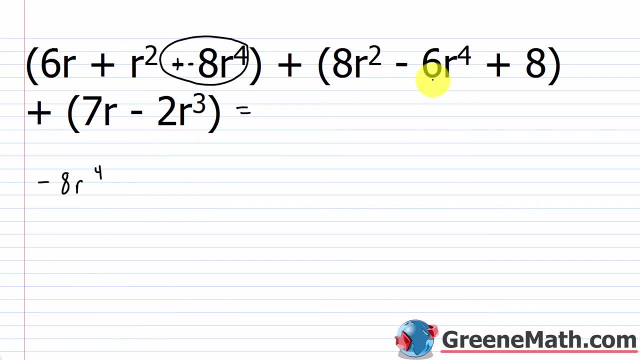 And then over here I see I have negative 6r to the fourth power. So I write those two next to each other Again. why did I start out with that? Because, as I scan through here, the highest exponent on r is a 4.. 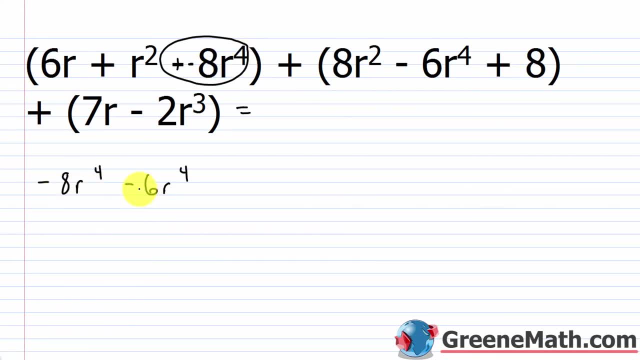 So that's why I chose to put this all the way to the left. Now I'm going to scan through and see: do I have r cubed? Yeah, I've got one right here. So again, the sign comes with it. 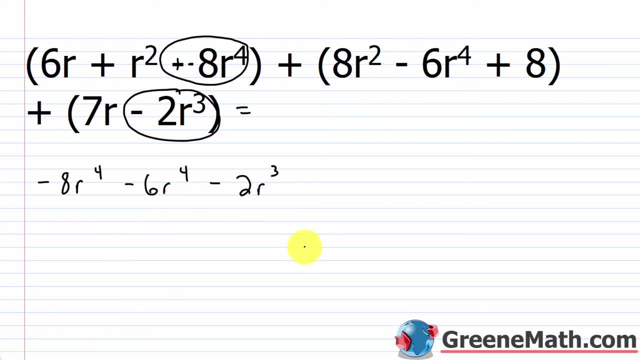 I'm going to write negative 2r cubed, And the next thing I'm going to look for is r squared. So I've got that here and here, So I'm going to put plus r, r squared, then plus 8r squared. 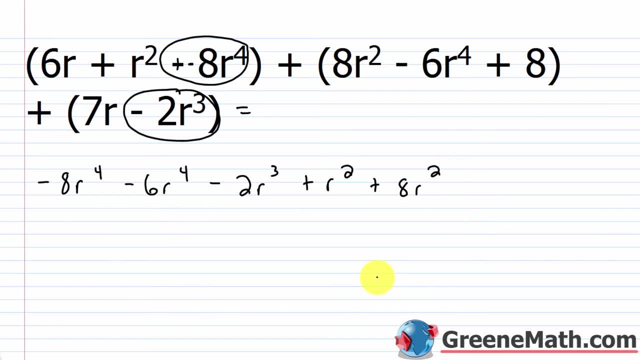 Now I'm looking for r to the first power, And so that's 6r and 7r. So plus 6r plus 7r. And then, lastly, I have this: plus 8.. So plus 8.. Now one of the things you might want to do, especially when you first start out. 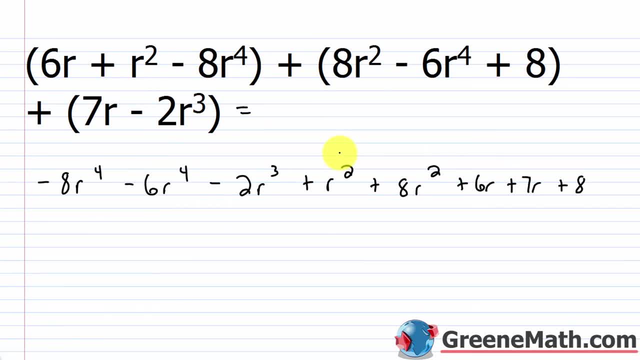 you might write everything and you might miss a term. Oh, I forgot that one. It's very, very common, So you can kind of go through, especially if you're on an important test, and check. Okay, I've got negative. 8r to the fourth power. 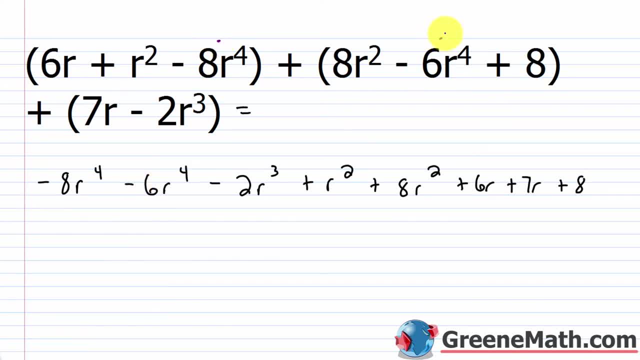 So I've got that Negative 6r to the fourth power. So I've got that Negative 2r cubed. I've got that r squared. I've got that 8r squared. I've got that. 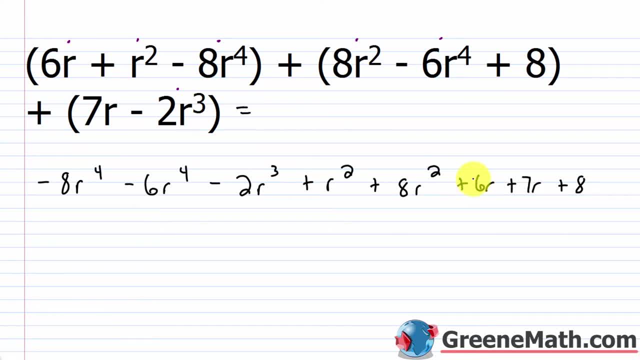 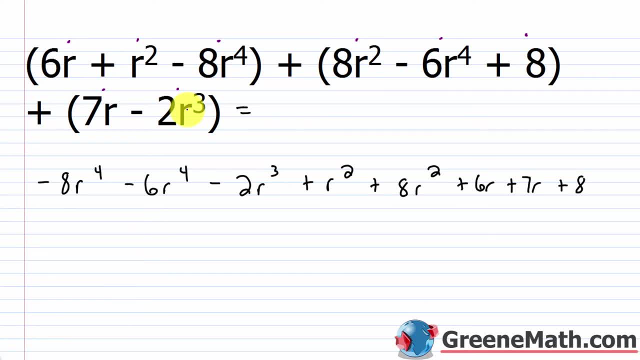 there, there. So I've got all my terms. So very important that you put everything in there, Otherwise you're not going to get the right answer. So once we've set this up, we're just going to combine like terms. 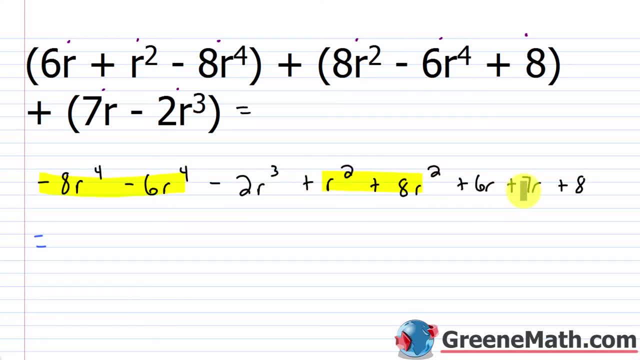 We've got like terms here and here and here. So negative 8r to the fourth power, minus 6r to the fourth power is going to be negative 14r to the fourth power. Then we've got minus 2r cubed. 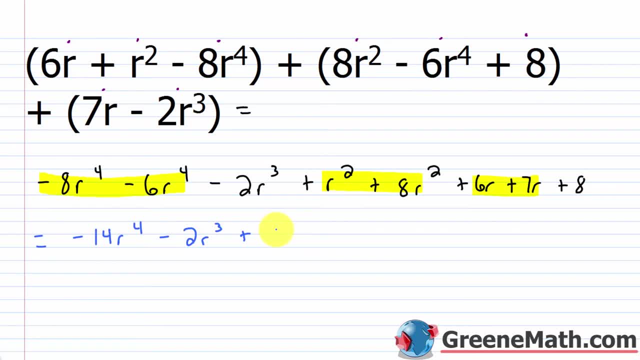 Then plus, you've got r squared plus 8r squared, which is 9r squared. Then plus 6r plus 7r is 13r, Then plus 8.. So it's just as easy as that And a lot of times moving forward. you're not even going to write this stuff out. 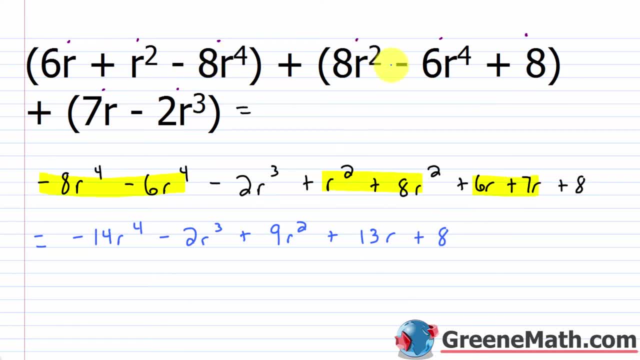 Once you get good at this, you're just going to say: OK, well, negative 8r to the fourth power, minus 6r to the fourth power, Write my answer negative 14r to the fourth power and just kind of go from there. 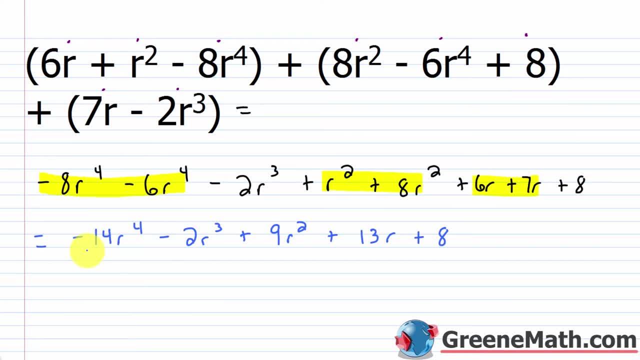 I add these now just kind of mentally and just write down the answer. I don't advise that until you get really good at this, Because it's very easy. It's very easy to make a mistake. So just start out with it, slow progress, until you fully understand it, and then you can. 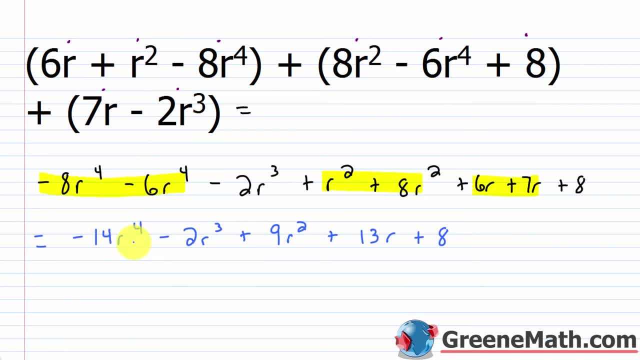 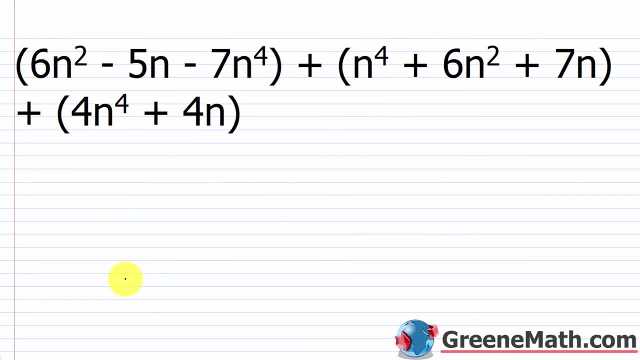 try to do it just a little bit faster. So our answer here is negative: 14r to the fourth power minus 2r cubed plus 9r squared plus 13r plus 8.. All right, so the next one is going to be 6n squared minus 5n minus 7n to the fourth. 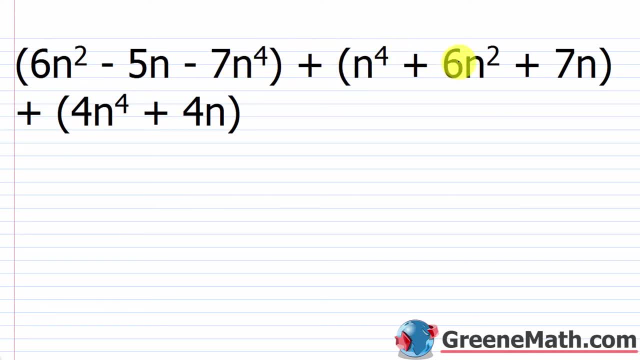 power. then plus n to the fourth power plus 6n, squared plus 7n, then plus 4n to the fourth power plus 4n. So I scan through this and I see that 4 is the highest exponent. So what has a 4 as an exponent? 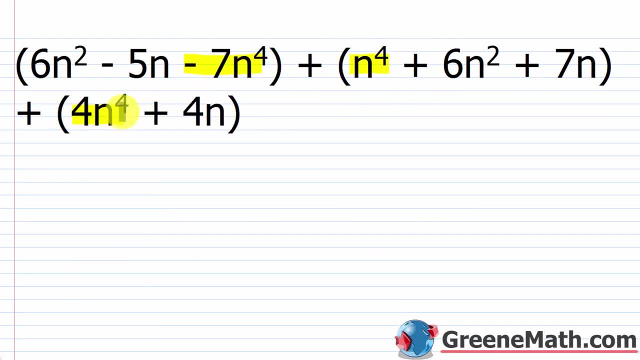 So this term, this term and this term, Let's put equals. I'll start out with negative 7n to the fourth power. Again, take the negative sign with you, Plus n to the fourth power. I'll do that next. 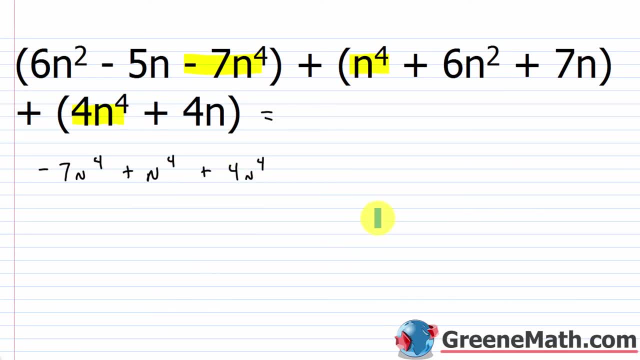 Then plus 4n to the fourth power. Now the next highest exponent would be a 2.. I've got 6n squared. I've got 6n squared again, and that's all I've got. Let's write those. 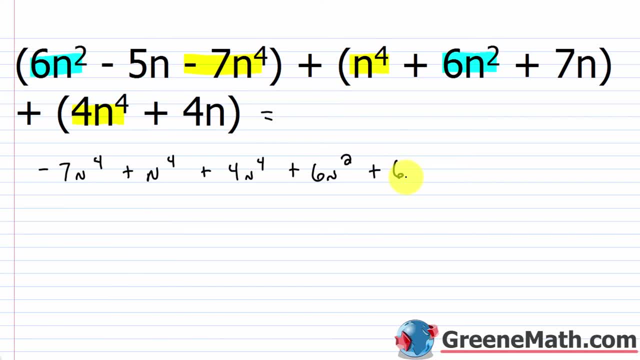 So plus 6n squared, plus 6n squared again, Then I've got my n to the first power. So I've got minus 5n and I've got plus 7n and I've got plus 4n. 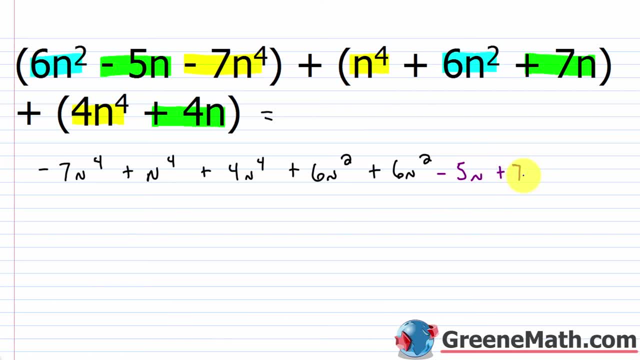 So let's go ahead and write those. I've got minus 5n plus 7n plus 4n, Okay, So now we're just going to combine like terms, And so I have like terms here. I have- let me do this in a different color- like terms here. 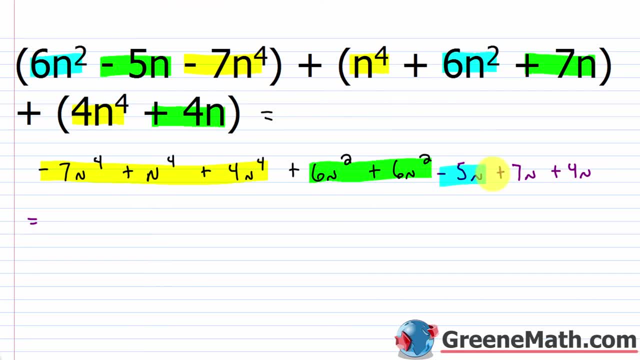 And then I have like terms. I'm going to switch colors again here. So if I look at it, what am I going to have? Negative 7n to the fourth power plus n to the fourth power, plus 4n to the fourth power. 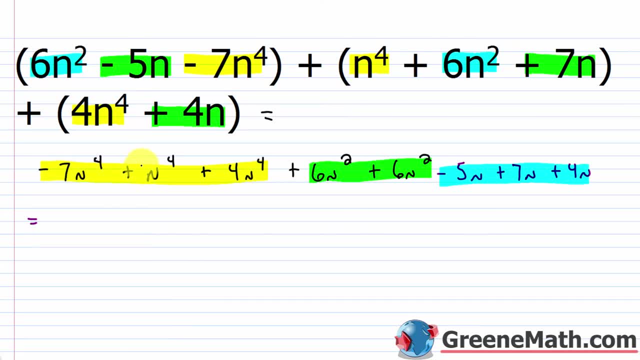 Just add the coefficients, So negative 7 plus this coefficient is understood to be 1.. So negative 7 plus 1 is negative 6. Negative 6 plus 4 is negative 2. This would be negative 2 times n to the fourth power. 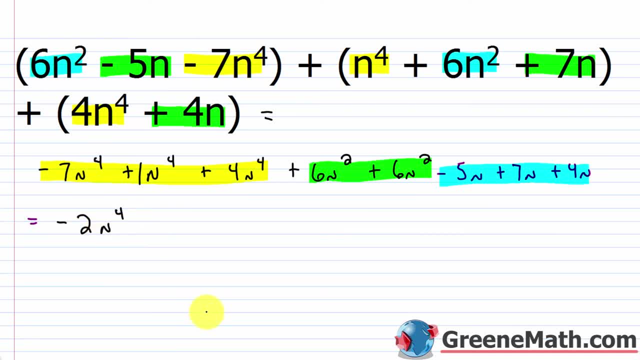 So I've got negative 7 plus 4n to the fourth power, plus 4n to the fourth power. Just add the coefficients. Negative n to the fourth power, just stays the same. Then plus, You have 6n squared plus 6n squared. 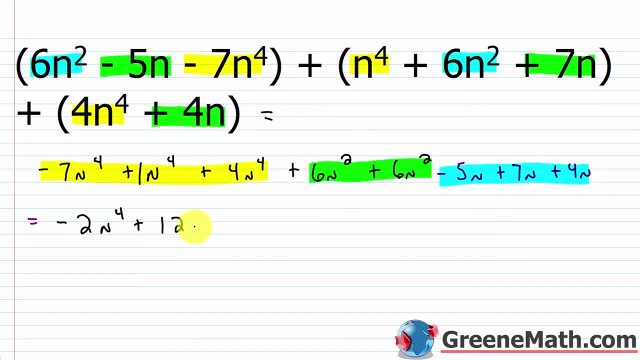 Do 6 plus 6,, that's 12.. Times: we have n squared. that stays the same. Then you have negative 5n plus 7n plus 4n. So you have negative 5 plus 7,, which is 2,, plus 4,, which is 6.. 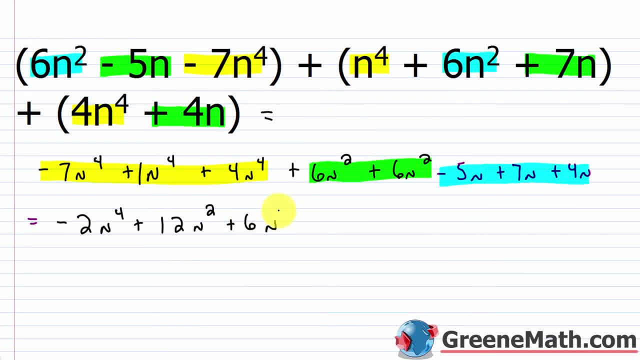 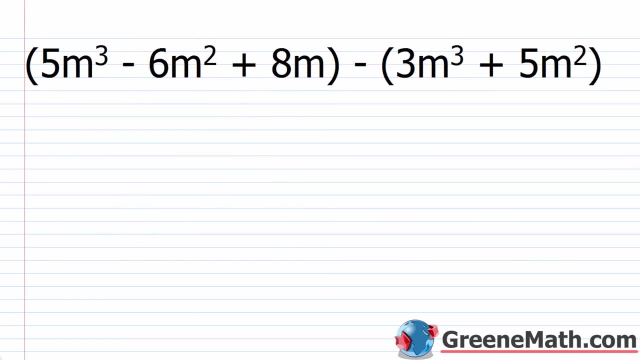 So plus 6 times n. So I end up with negative 2n to the fourth power plus 12n squared plus 6n. All right, get into some subtraction problems. and subtraction is not any more difficult than addition. you just have to know one thing: whatever polynomial is being subtracted away, what you want to do is: 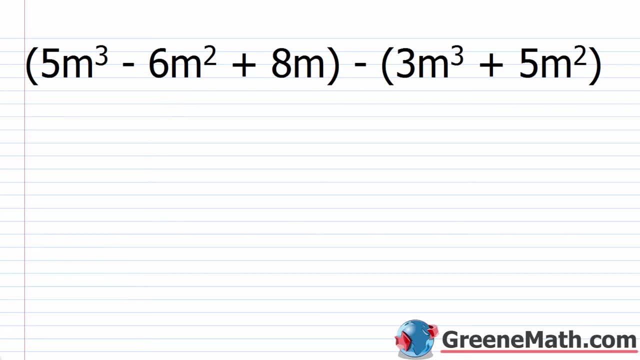 you want to change the sign of each term of the polynomial being subtracted away and then you just add: so, as an example, we have 5m cubed minus. 6m squared plus 8m, then minus, we have 3m cubed plus. 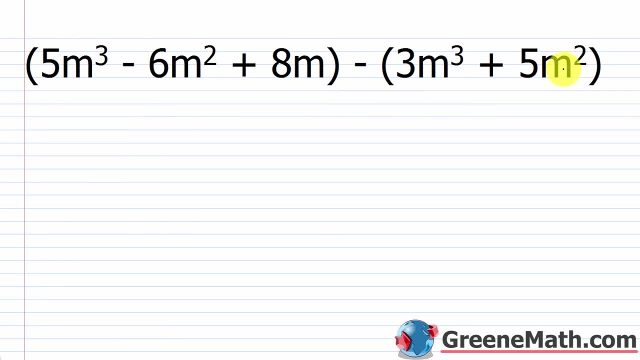 5m squared. now a lot of students get confused and they're like: well, what's the difference between having this minus 6m squared and minus this whole thing? here the difference is i have a minus sign outside of this set of parentheses, so this whole thing is being subtracted away. so if i'm 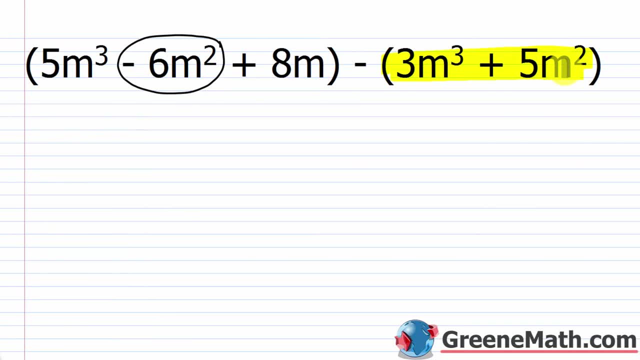 subtracting the whole thing away. what i can do- and you'll see a lot of professors do this- you'll see plus negative one there and they'll distribute the negative one to each term just as a reminder to the student to change the sign of each term and then just add so, in other words, if i do it this way, i'd 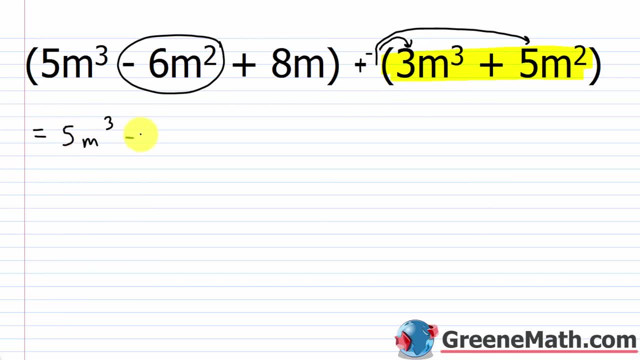 rewrite this problem as: 5m cubed minus 6m squared plus 8m. negative 1 times 3m cubed is negative 3m cubed, and then negative 1 times 5m squared is minus 5m squared. so again, all i'm doing is i'm. 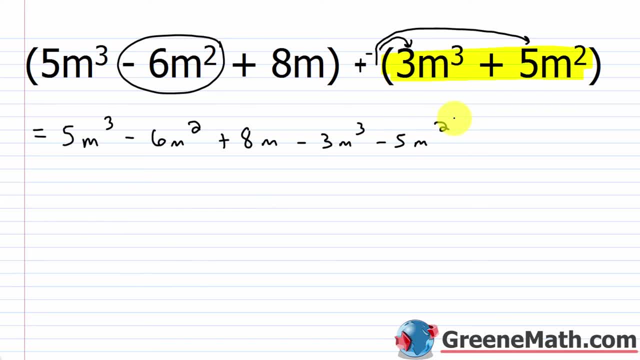 changing the sign of every term in the polynomial that's being subtracted away. i could have just as easily said: okay, i've got minus 3m cubed and then minus 5m squared. where students make another mistake is they'll drop the parentheses. they'll say: i have minus 3m cubed. they got the first term. 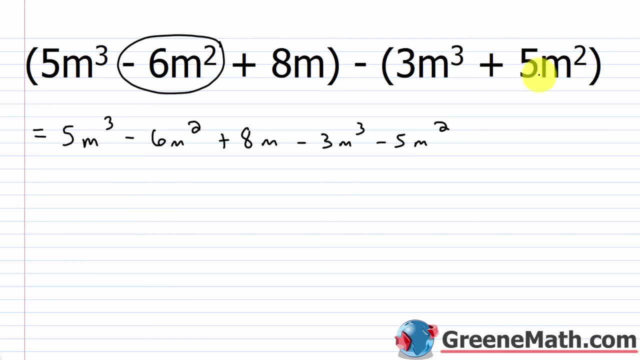 right. but then the second term they forget to change. they just leave that as plus 5m squared and they get the wrong answer. you need a minus here and here. okay, very important. so once you have that, you just combine like terms, like we've been doing with addition. okay, so it's. 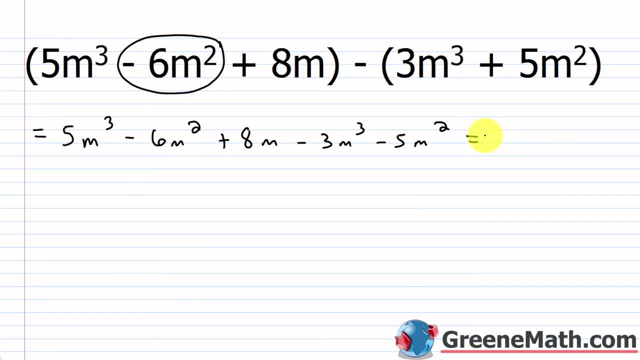 just one additional step and to kind of look at this, i would write 5m cubed all the way to the left and then minus 3m cubed- those are like terms- and then minus 6m squared and then minus 5m squared. 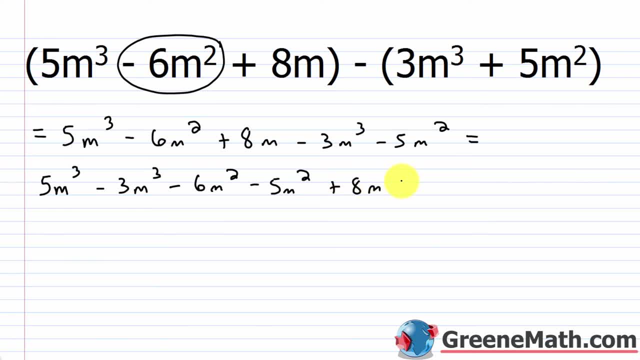 those are like terms, and then plus 8m. so 5m cubed minus 3m cubed is 2m cubed. negative 6m squared. minus 5m squared is negative 11m squared. and then i have plus 8m. so again my 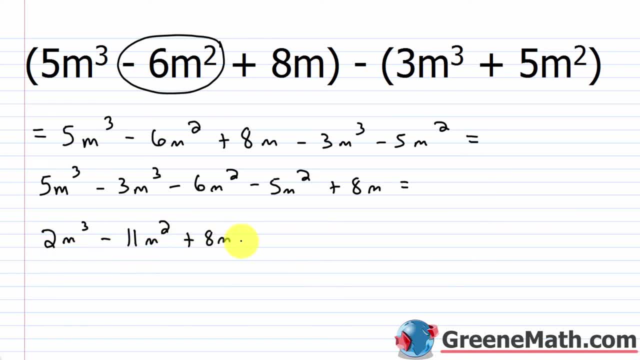 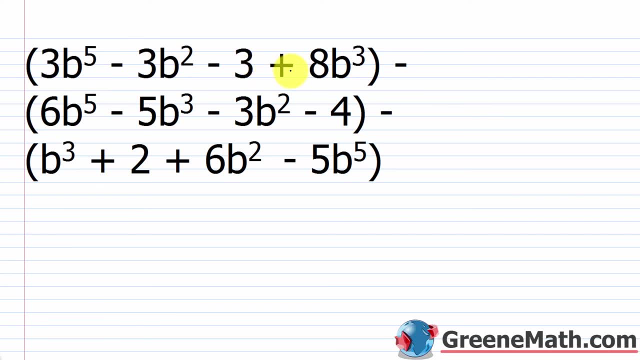 answer here is 2m cubed minus 11m squared plus 8m. all right, let's take a look at another one. so we have 3b to the fifth power minus 3b, squared minus 3, plus 8b cubed, then minus. 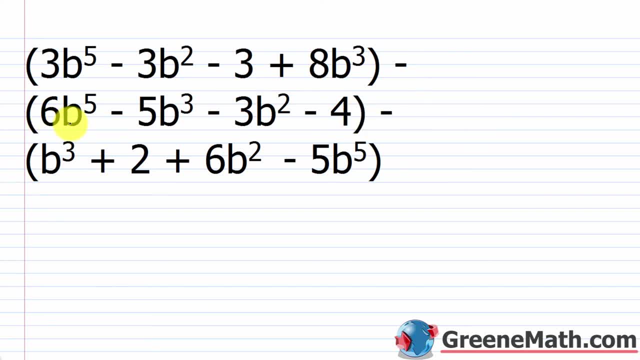 we're subtracting away this whole polynomial here: 6b to the fifth power minus 5b cubed, plus 3b squared, minus 4, then minus. i'm subtracting away this whole thing: b cubed plus 2 plus 6b squared. 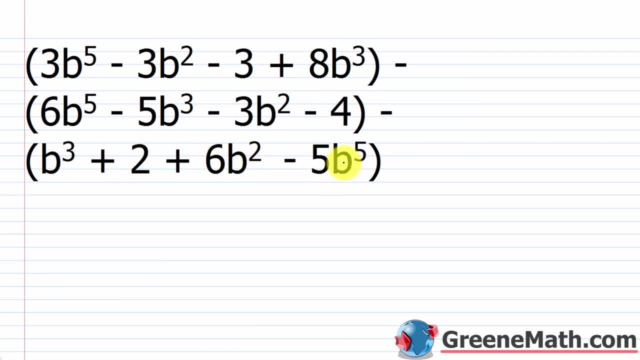 minus 5b to the fifth power. now, the quickest thing you can do again, you can just make this plus and change every sign here. so this would be negative. this would be positive, positive, positive. change the sign here: plus negative. this would be negative, negative, positive. okay, change the sign of every term that's being: 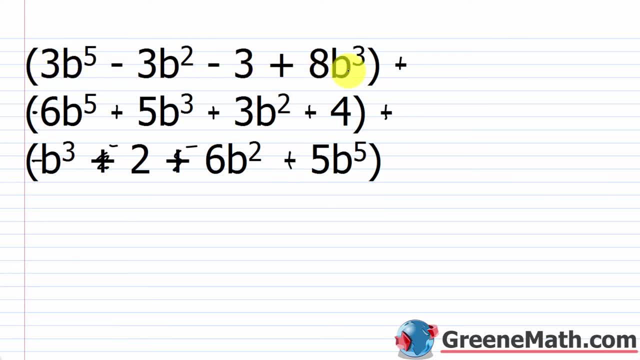 subtracted away. this first polynomial is not being subtracted away, so it just stays as it is. every polynomial that comes after it has a subtraction sign out in front of the parentheses that enclose it. so you've got to put a plus sign and then change every sign for the terms inside the 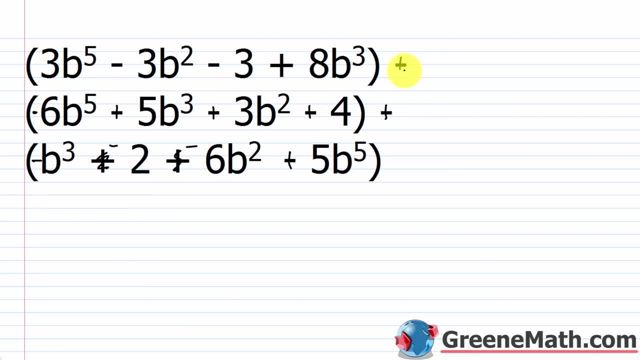 parentheses. okay, very important, you understand that. and again, if you struggle with it, put plus negative one and distribute the negative one to each term. it's going to remind you to do that. all right, so what i'm going to do here. if i scan through, i see 5 is the highest exponent. 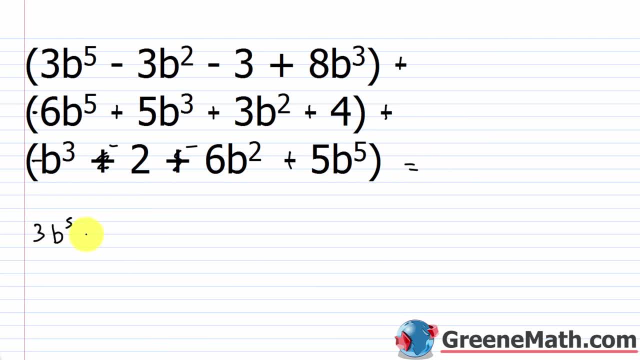 so i've got 3b to the fifth power. i've got negative 6b to the fifth power and i've got 5b to the fifth power. so that takes care of this one, this one and this one, and the one that's in the highest i see is a three. so i've got 8b cubed. i've got 5b cubed. 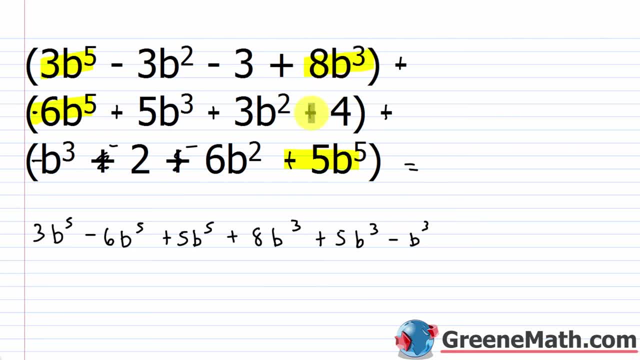 and i've got negative b cubed. okay, so that takes care of this one, this one and this one. all right, so the next thing i see is b squared. so i've got a negative 3b squared. i've got positive 3b squared, negative 6b squared. so that's going to take care of this one, this one and this one, and then lastly, 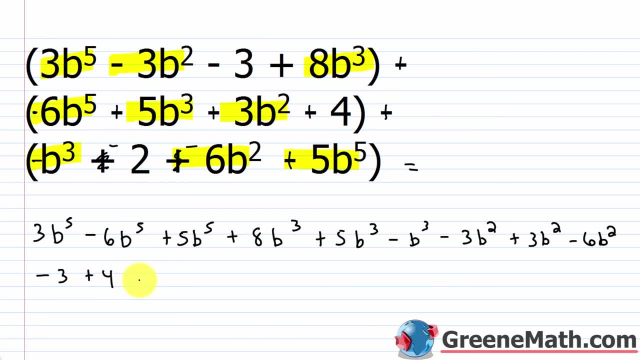 i have minus three, i have plus four and i have minus two. so that takes care of this one, this one and this one. and because i've highlighted everything, i know i didn't miss anything. and again, it gets very, very tedious with these kind of longer problems, so you need some kind 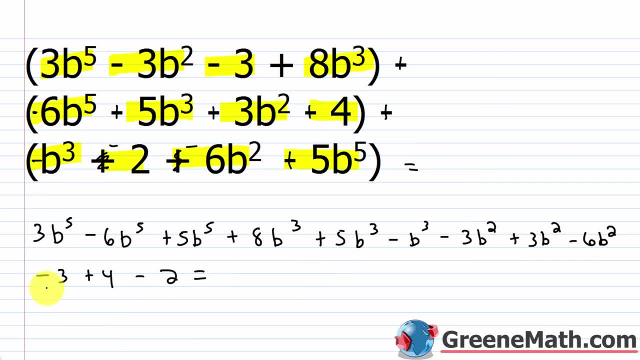 of process to tell you, hey, i've used all of these. so if i start with 3b to the fifth power, minus 6b to the fifth power, plus 5b to the fifth power, again look at your coefficients. 3 minus 6 is 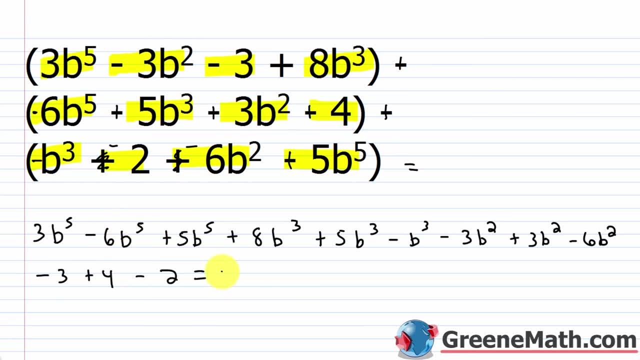 negative. 3 plus 5 is 2, so i've got 2. and then times b to the fifth power. here i've got 8b cubed plus 5b cubed, minus b cubed. again i've got an 8 a 5, and this would be a negative 1. 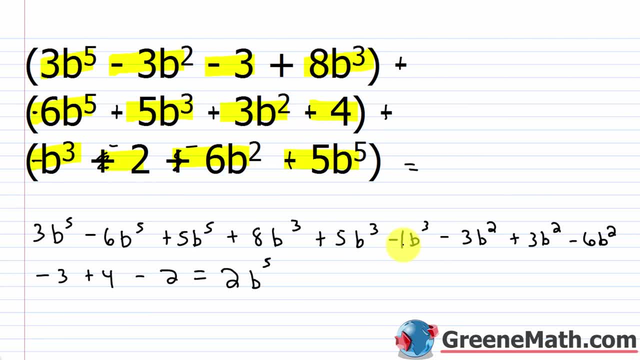 understand that if you have a variable by itself, the coefficient is one. If you have a negative in front of it, the coefficient is negative one. You can't just not put anything. So for this, one eight plus five is 13.. 13 minus one is 12.. So this would be plus 12b cubed. Then next I have negative three b. 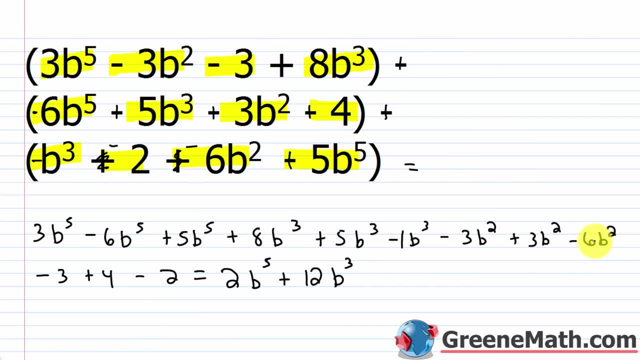 squared plus three b squared, minus six b squared. So I think about negative three plus three is zero, Those are opposites. And then I just have negative six b squared, So minus six b squared. And then, lastly, I have negative three plus four, That's one, Then minus two is negative one. So 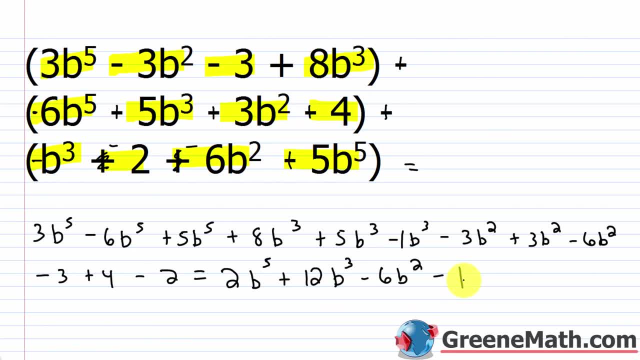 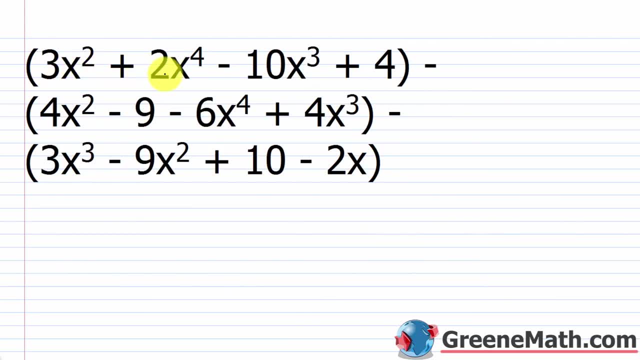 minus one. So two b to the fifth power plus 12b cubed minus six b squared minus one. All right, the next thing I want to look at is three x squared plus two x to the fourth power minus 10x cubed plus four. Then minus this polynomial, here We have four x squared. 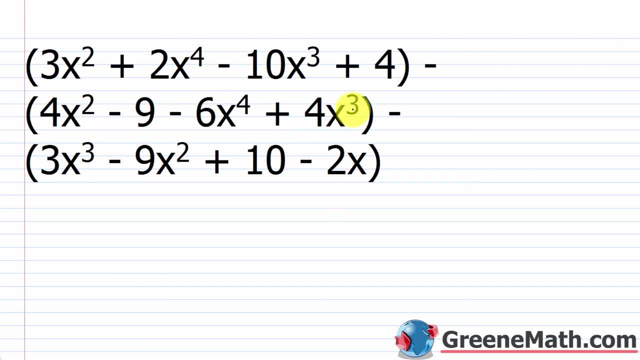 Minus nine minus six x to the fourth power plus four x cubed, Then minus, I have three x cubed minus nine x squared plus 10 minus two x. Again, this first polynomial is just going to stay the same. So just my three x squared plus two x to the fourth power, minus 10x cubed plus four. 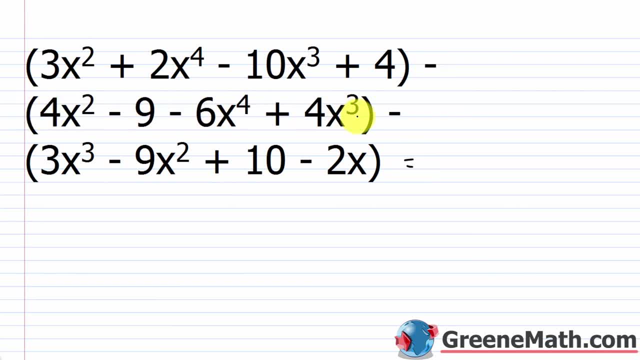 I'm subtracting away this polynomial here, So all I want to do is put plus and then change the sign of each term, So this becomes negative, positive, Positive, And then this would be negative For the next one. it's the same. I'm subtracting. 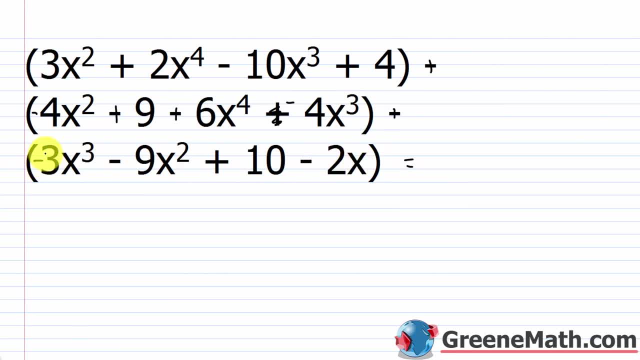 away this polynomial here. So plus This is negative, Positive, Put negative And then positive. All right. So once we've done that, I'm going to scan through. I see four is the highest exponent. So I've got two x to the fourth power. I've got six x to the fourth power. 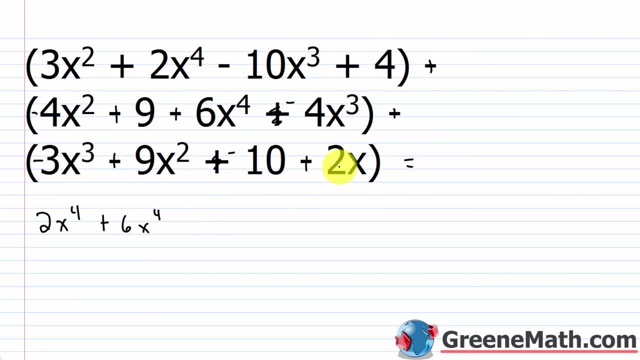 And I don't have an x to the fourth power here. So that just takes care of this and this. Now next I scan through and I see x cubed. So I see I have negative 10x cubed, So minus 10x cubed. Then I have minus four x cubed, And then I have minus three x cubed. So that takes. 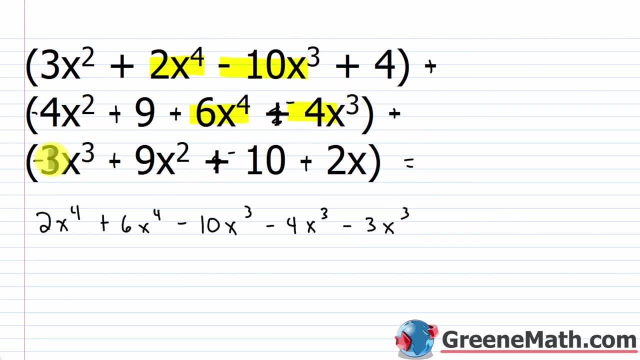 care of this, this and this, The next. I see I have x squared, So I have plus three x squared. I have minus four x squared, And then I have negative 10x cubed, So I have minus three x cubed. 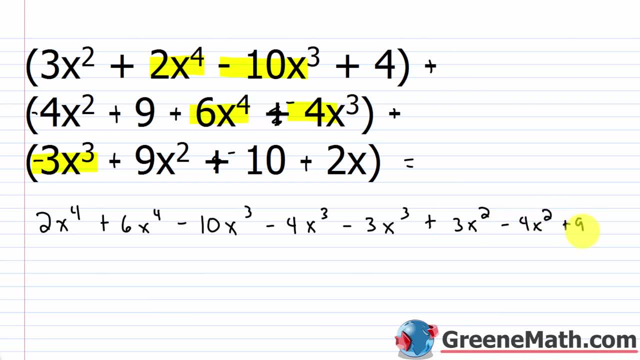 And I have plus nine x squared. So that takes care of this, this and this. All right. So, lastly, I have this: two x, So that takes care of this. No more x to the first power anywhere. And then I. 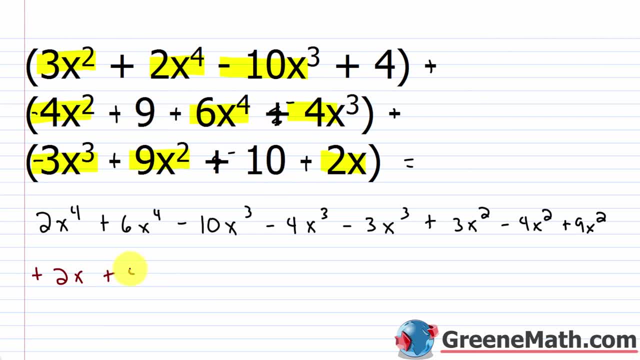 have four, nine and negative 10.. So plus four plus nine, plus negative 10, or minus 10.. Whatever you want to do, All right, So that takes care of this. And then I have plus nine and negative 10.. 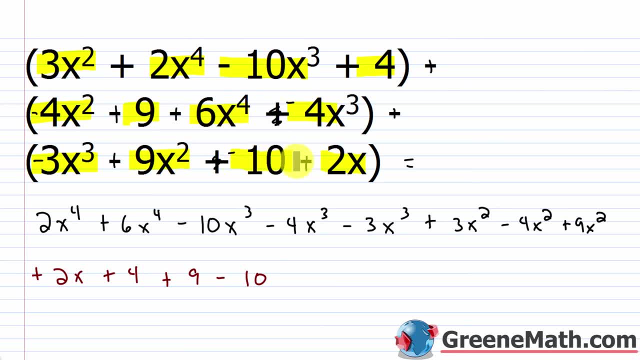 Whatever you want to do, All right. So that takes care of this, this and this. And again, notice how I've highlighted everything, so I know I didn't miss anything. Okay, So I go through now and I say: two x to the fourth power plus six x to the fourth power. Two plus six is eight times x.